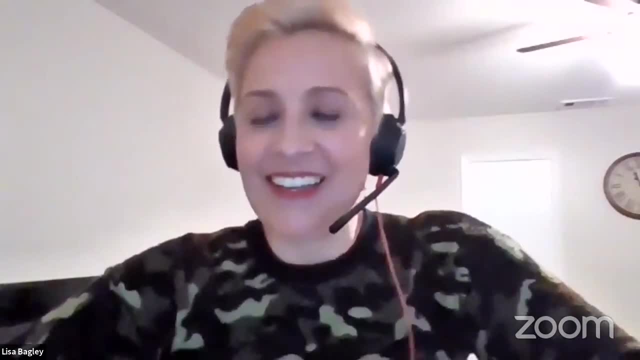 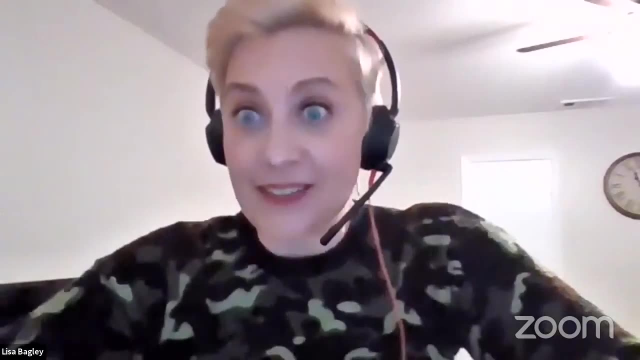 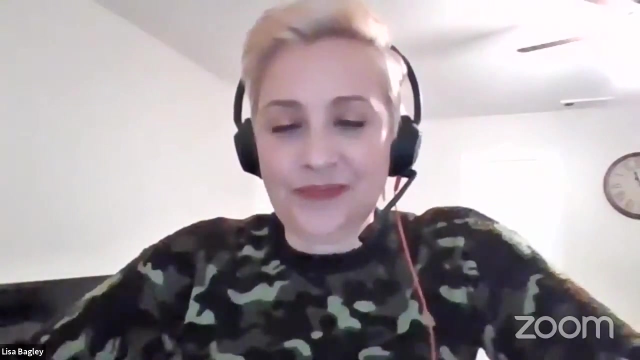 Hey everyone, Welcome back. It is day three. AP Daily Live. AP Environmental Science. Thanks for being here for the third day in this series. I'm going to go ahead and start my screen, So before we get started, let me reintroduce myself. My name is Lisa Bagley. 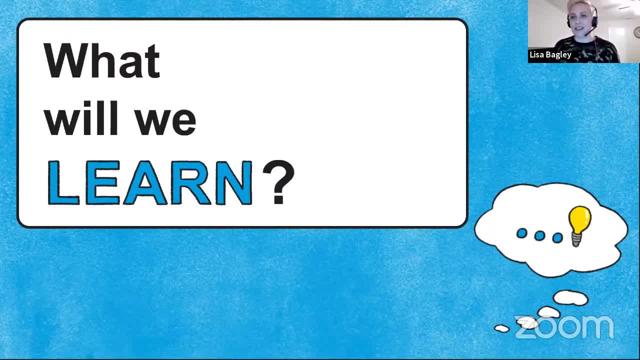 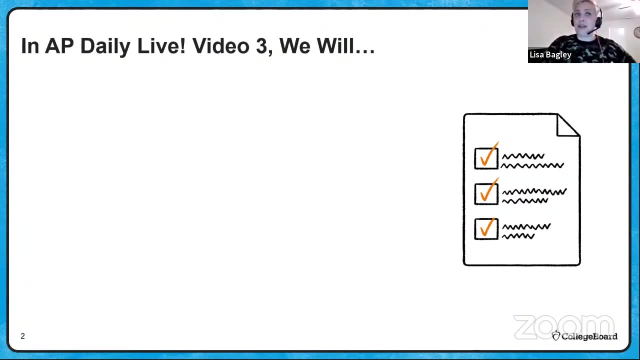 I teach in Texas, right outside of Dallas Mesquite ISD. Go Wranglers. What are we going to learn today? Well, funny, you should ask on this Earth Day Eve. In AP Daily Live video three, we're going to answer questions and provide clarification of. 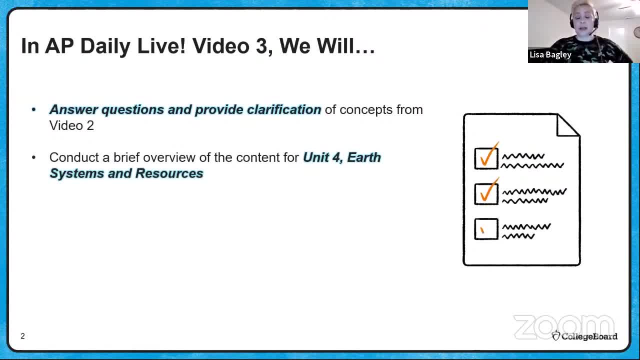 concepts from video two. We're going to conduct a brief overview of content for unit four: Earth Systems and Resources. We're going to practice connecting our free response questions to answers- free response question answers to the science practices in order to maximize score. 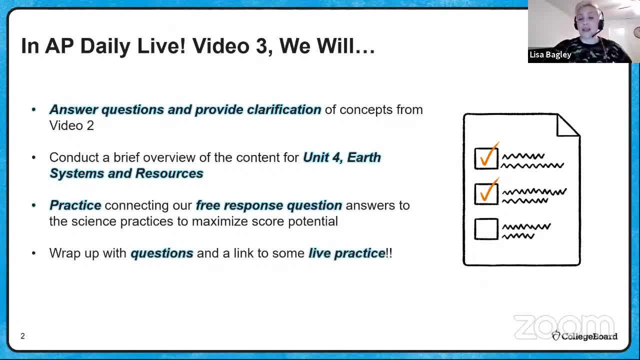 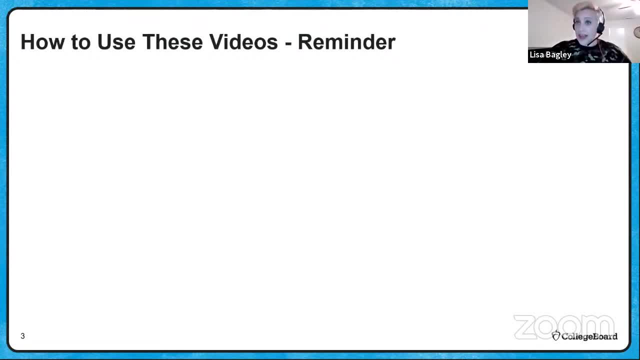 potential And we're going to wrap up with questions and a link to some live practice. Just a reminder on what these videos are for and how to use them. AP Daily Live videos are designed to help you understand how to demonstrate your environmental science content knowledge. 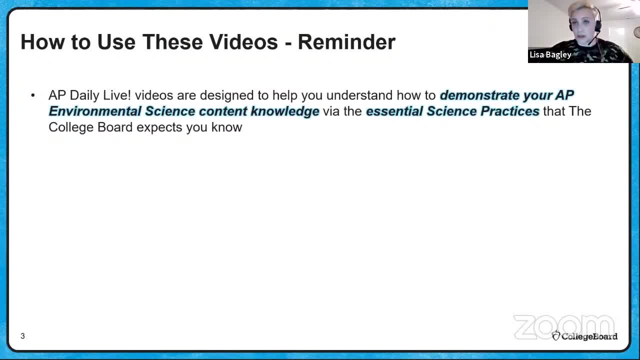 via the essential tools of the science. So if you're interested in learning more about the essential science practices, the College Board expects you to know. These are not specifically content review videos. However, the AP Daily content videos that are presented in the units. 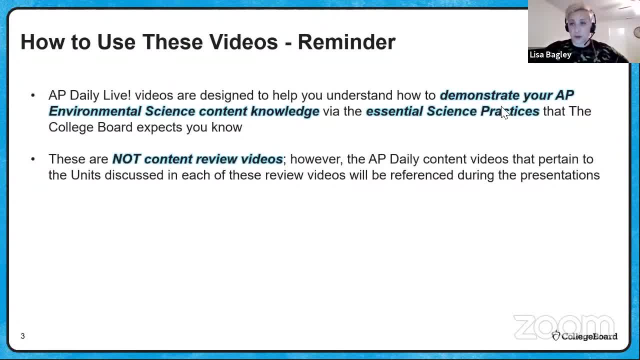 discussed for each of the review videos will be referenced during the presentations. I want to clarify that just a little bit. For this particular unit and whatever unit we're talking about, this happens to be unit four. If the content pertains to unit four, I will not reference. 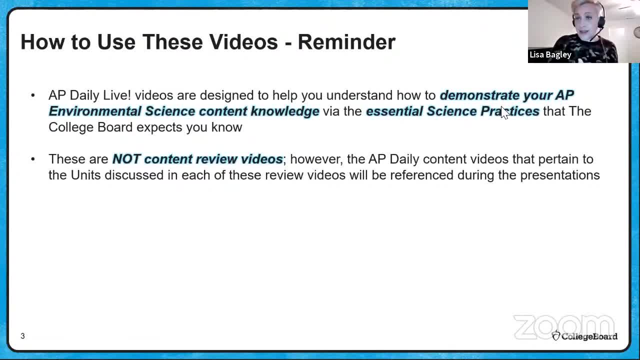 that video because those are those videos. If the content pertains to unit four, I will not reference that video because we have just gone over that content. But if the content comes from outside of the unit four videos, then those videos will be referenced During the free response question. 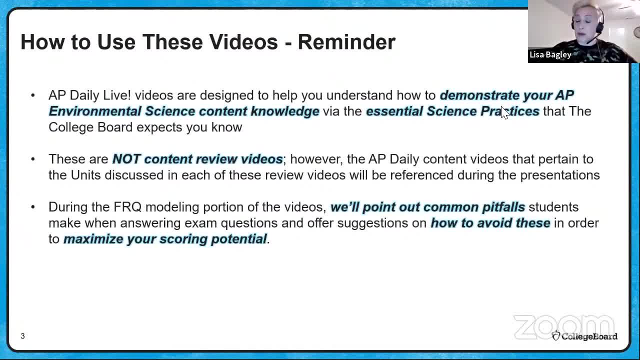 modeling portion of the videos, I'll point out common pitfalls that students often make when answering these exam questions and offer suggestions on how to avoid these and to maximize your scoring potential. And, as always, the videos are best used in conjunction with individual review on your own time, because, of course, you know better than I do. So if you're. 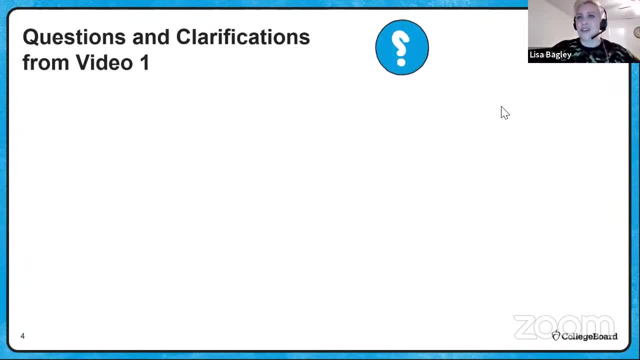 going to be doing a review. you're going to want to make sure that you're doing the best, what you need to work on. So first let's jump into questions and clarifications from this should say video two. This would be a video two clarifications. So again, I want to thank everybody. Y'all are 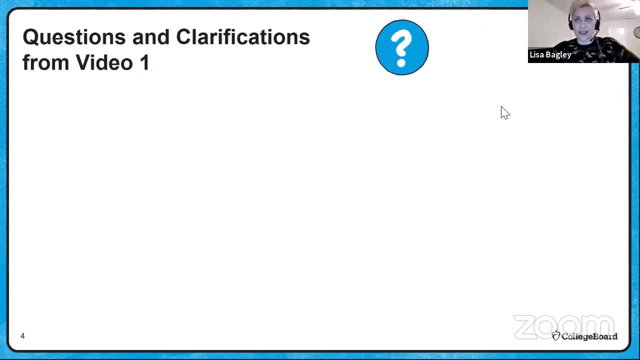 really amazing when it comes to giving feedback and suggestions, Like it's really really good And I want to give a shout out to everybody about that. So the first one I want to hit is: can you go over the format of the exam please? 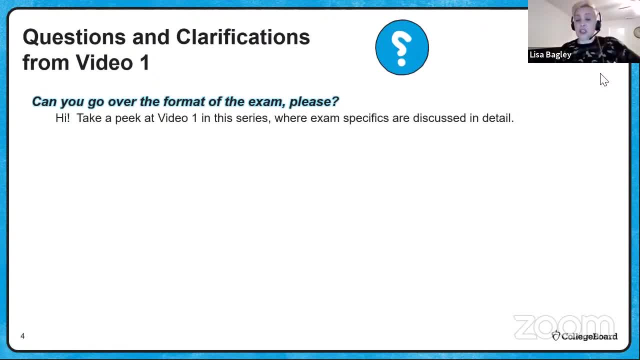 Well, thanks for asking. We did that back. in video one of the series, The exam specifics were discussed in detail. So if you still need to figure out what is going on with the specifics of the exam, please take a look at video one. The first part of that video does talk about that in. 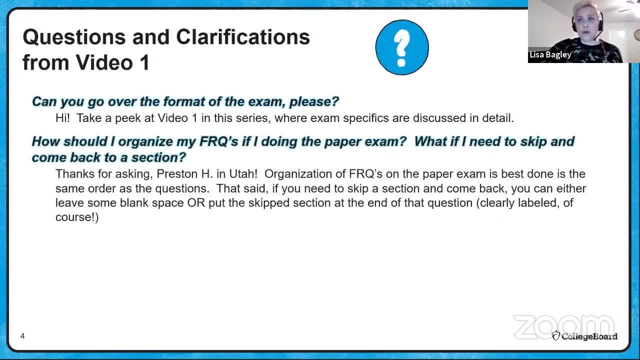 detail. All right, Several of you were questioning about if I'm a paper test taker, how do I organize my free response questions And what if I need to skip and come back to a section. So shout out to Preston H from Utah for asking that question: The organization of free response. 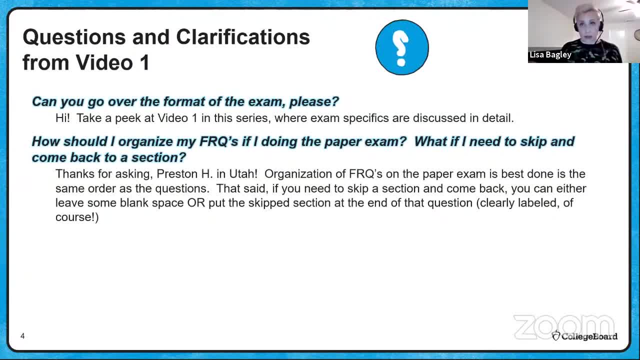 questions on the paper exam is best done in the same order as the questions. So, for example, if you're answering question prompt A, putting prompt A, putting the A in parentheses and then answering it, that's the easiest way for a reader to figure out what you're talking about and where. 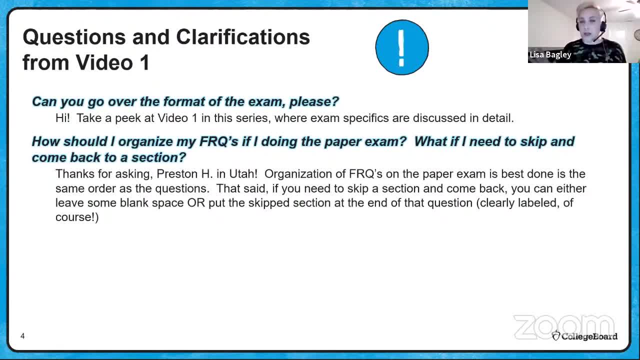 your points are, However. that said, if you need to skip a section and come back, you can either leave some blank space and then come back and write there, or you can put the skipped section at the end of your answer to that question, But make sure you label it. It just makes. 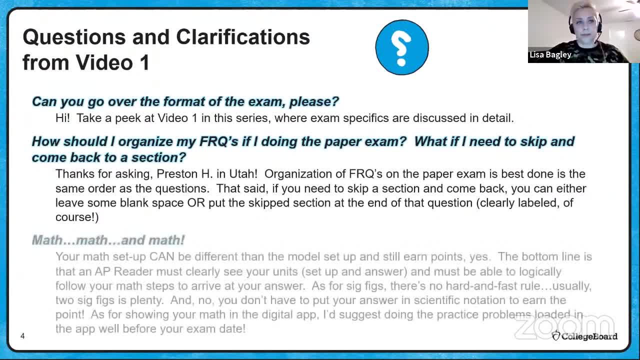 it easier for us to find your points when we're scoring it. Math, math and more math. Lots of questions about the math. So can my math setup be different than the model and still earn points? The answer to that is yes, it can. The math setup can be different and you can still earn points. 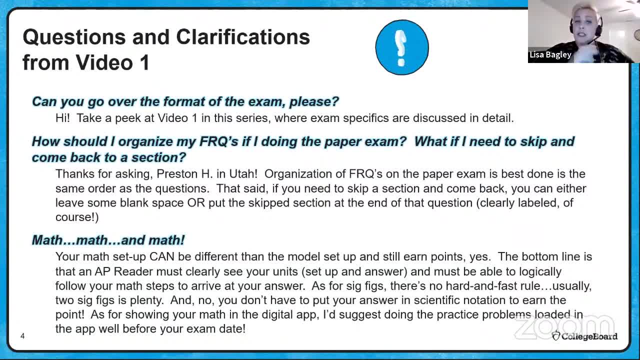 But the bottom line is that your AP reader must clearly be able to see both your units in the setup and the answer and they must be able to logically follow your math steps to arrive at the answer that you've given there. If the math is not like, if the math is not followable, is that even a word? If the 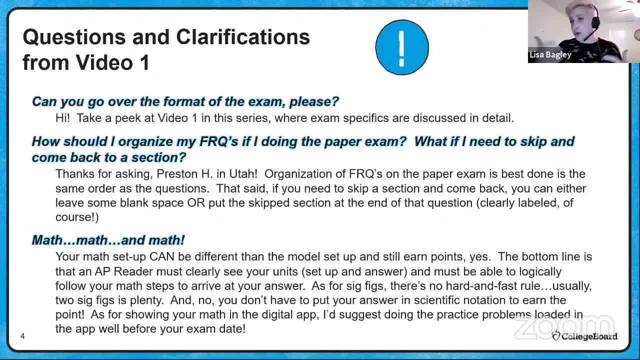 math is not followable or you don't have what's required, which are units in setup and answer, then it would not be pointable. Several of you asked for significant figures. As for sig figs, there's no hard answer. If you have a hard answer, you can ask for a significant figure. 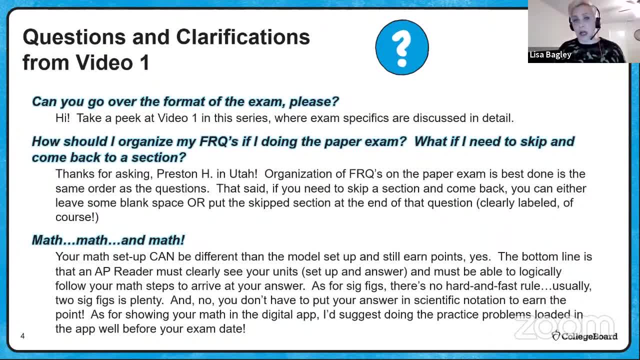 If you have a fast rule- usually two sig figs is plenty on the APES exam. And no, you do not have to put your answer into scientific notation. Several of you guys were like, hey, I have this in non-scientific notation because scientific notation freaks me out. Cool, It doesn't matter. 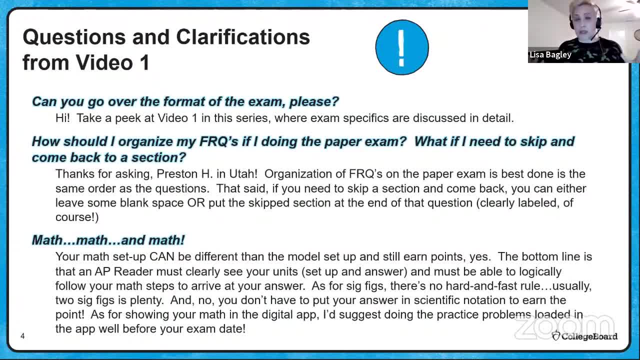 As long as it's the same answer as we would get with scientific notation, no problem whatsoever. It just makes it easier for us to look at sometimes, but still pointable. Several people asked about how do I show my math? So here's the deal with the digital app. You've got the practice app there, So one of the things 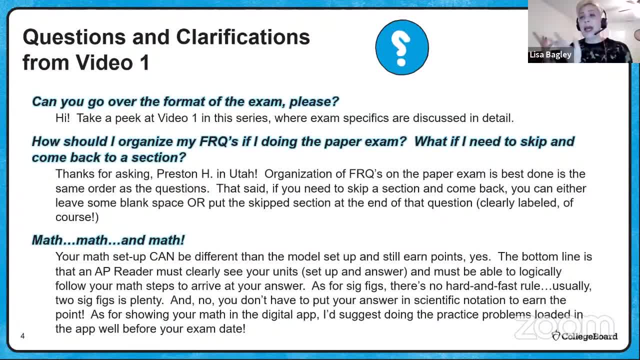 with the practice app is that they have practice problems that are loaded there, And I'm going to really highly suggest, like really suggest, that you guys practice in your digital app, putting those math equations in there, just to see how you do it. There's nothing in APES that can't be done. 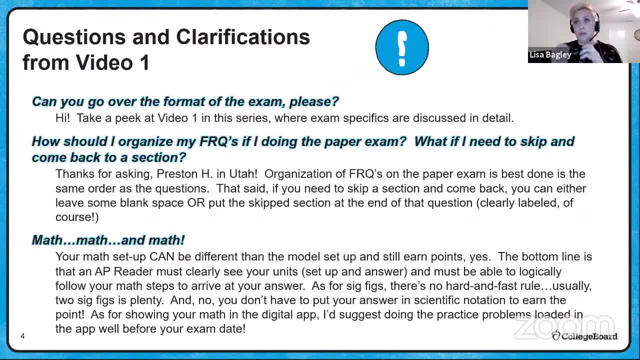 on a keyboard in terms of math And of course you know you're going to be able to type your units or whatever. So you've got a mixture of, you know, keyboard commands like the divide sign or the multiplication, the star for multiplication. You should be able to do all of that, but 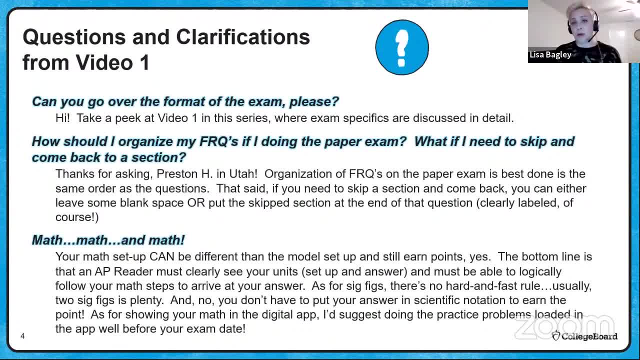 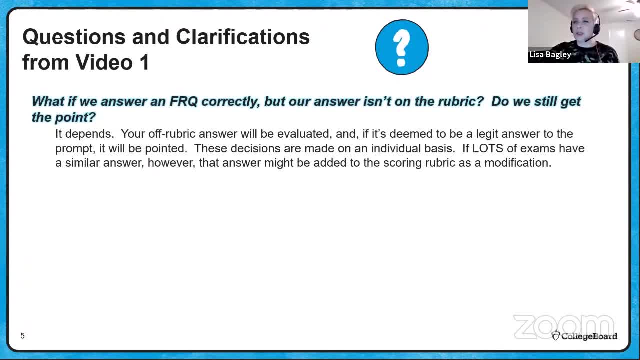 practice, practice so you're not going in cold, All right. So if we answer a free response question correctly but the answer isn't on the rubric, do we still get a point? Good question, And the answer to that is: it depends. 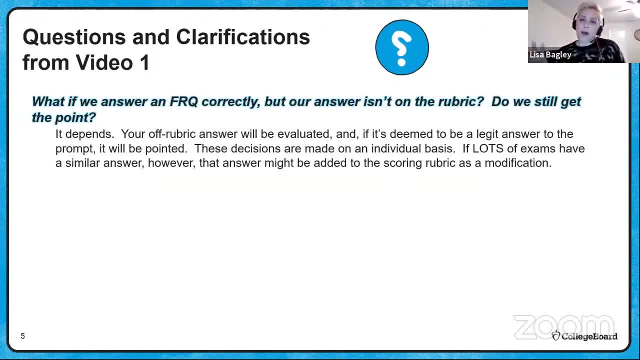 So if you have an off rubric answer, we'll evaluate it during the reading And if it's deemed to be a legitimate answer to the prompt right, then it's up to the question leader as to whether or not that will be pointed. The decisions are actually made on an individual. 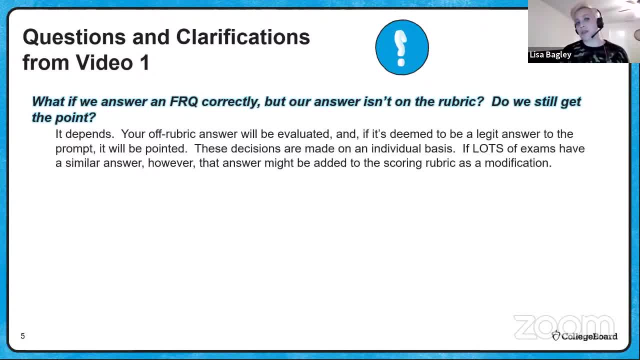 basis. However, if lots of examinations have a similar answer, then that answer might actually be added to the scoring rubric as a modification. So, generally speaking, if you have an off rubric, the rubric is set, but there is some wiggle room. if there is an FRQ answer, that fits but it hasn't. 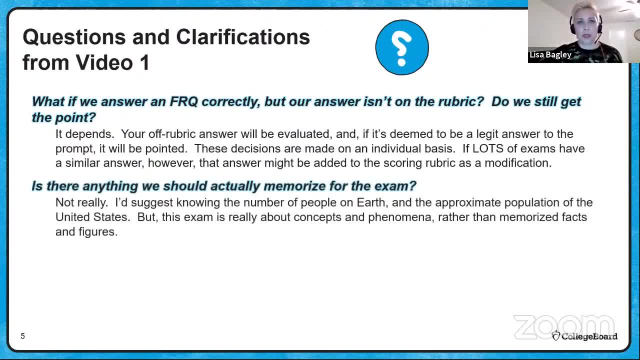 been identified on the rubric. That's fairly rare. however, Is there anything we should actually memorize for this exam? This exam is not really high on memorization. I would suggest knowing some basic stats, like how many people are on earth and what's the approximate population of. the United States. But in general this exam is not really high on memorization. So if you have some basic stats like how many people are on earth and what's the approximate population of the United States, then that's very small. But if you have some basic stats, then that's rather high on. the rubric. This exam is not really high on memorization. So if you have some basic stats, Then the answer is yes, that is correct. That is correct. If you have some basic stats, then yes, that is correct. 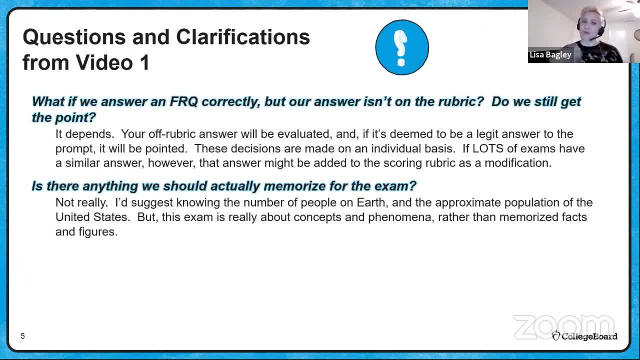 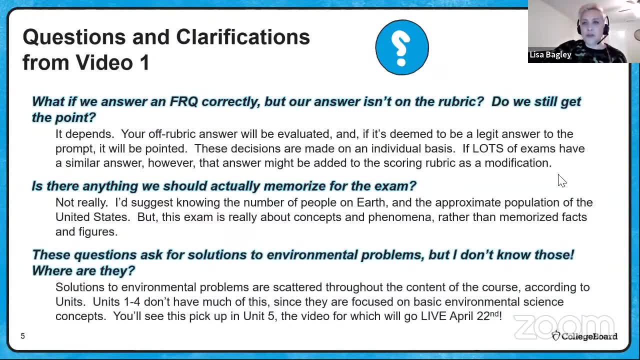 If you have some basic stats, then yes, it's correct. Okay, if we're going to review this with a review of in, then let me know the answer, because I'm just wondering if you have any kind of experience where you can do an initial review. 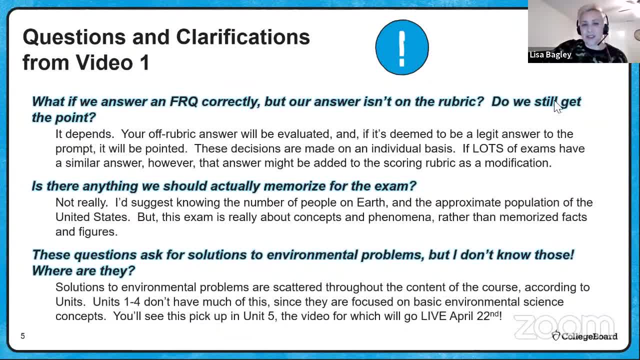 of the results and make some decisions based on a particular question that you have. I want to make sure that the answer is true. I'm going to go back to a little bit of my area of expertise. This is an example of how, but I don't know these solutions. Where are they? Well, the solutions to environmental problems are: 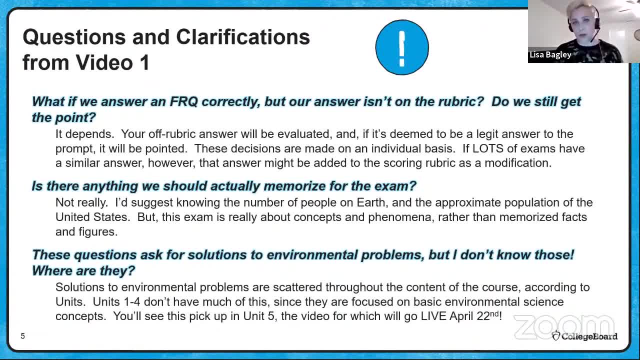 kind of scattered throughout the content of the course and that's according to unit. So just a caveat: units one through four don't have a lot of solutions to environmental problems and that is because of the nature of units one through four. They're mostly focused on basic environmental. 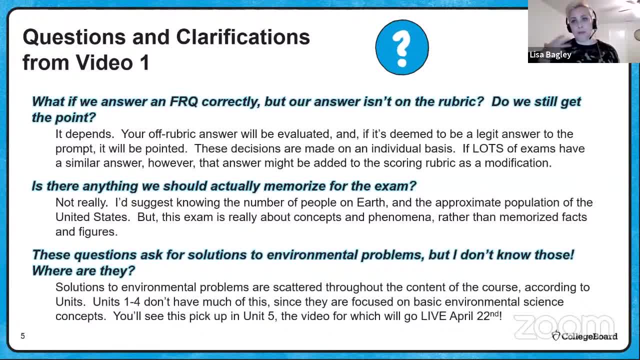 science concepts, right. So the make a claim you'll see in a lot of these models. the make a claim comes from other units. in these first few units, because there's not a lot of make in a claim- you're going to do with certain ecology concepts or systems concepts. You're going to 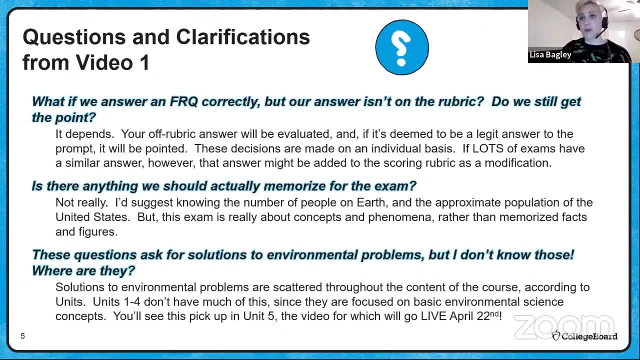 see this, pick up a lot in unit five and continue on through the rest of the videos throughout the rest of the course, and unit five is going to be covered tomorrow in our live session on April 22nd, So you're going to see how that. 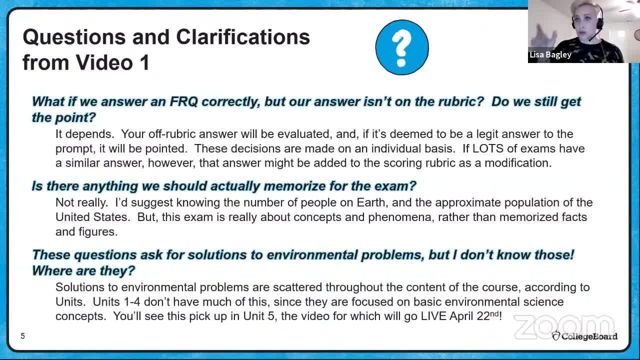 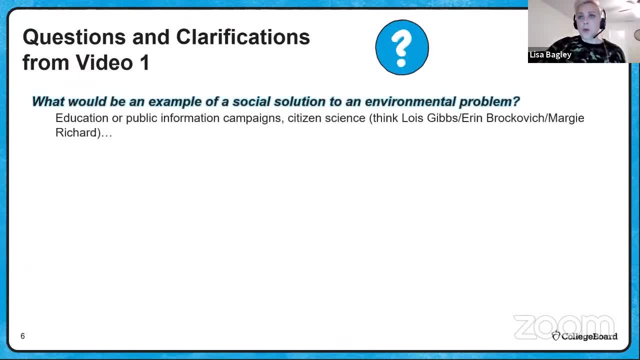 unit five is going to be covered tomorrow in our live session on April 22nd. So you're going to see how the content of that unit lends itself to environmental solutions and I'll point that out specifically. All right, So what would be an example of a social solution to an environmental 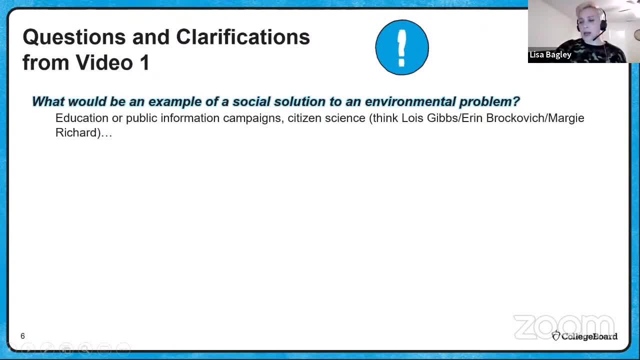 problem. I had mentioned that you need to make sure that you're actually answering the type of solution that they're asking for. Well, good question. You could have an education or a public information campaign, citizen science initiatives like what the Lois Gibbs did with Love Canal or Erin Brockovich in Hinkley, California with you know, toxic waste. 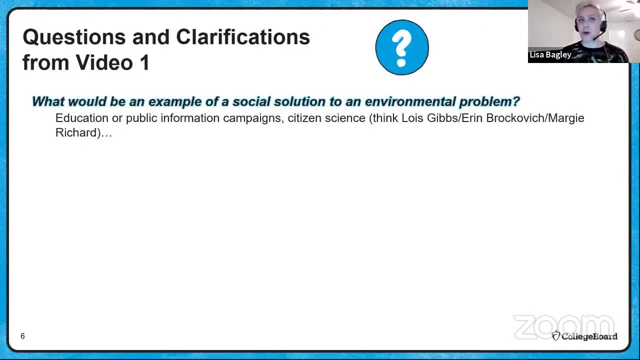 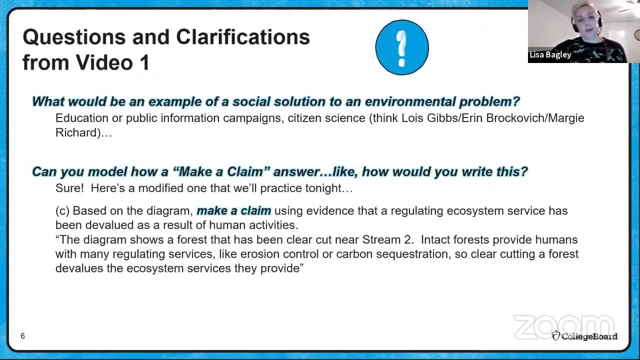 dumping, or Margie Richard in Norco, Louisiana. So if you don't know who those people are, those are great case studies. You might want to look them up. Hey, Ms Bagley, can you model how a make a claim? answer would look if you were to write it. Thank, 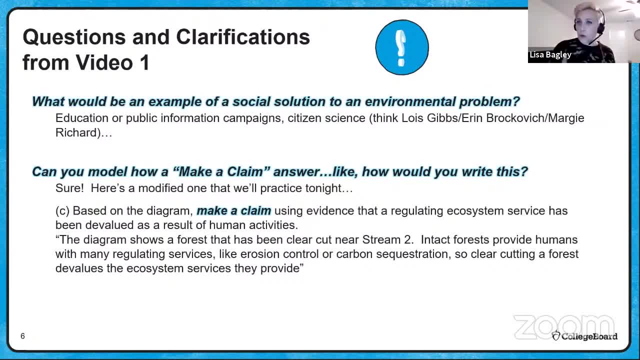 you for asking. In these videos I've just kind of been giving you what the rubric prompt would look like. but I haven't been able to figure out what the rubric prompt would look like, So I'm going to model exactly what a student response might look like. So we're going to talk. actually we're going. 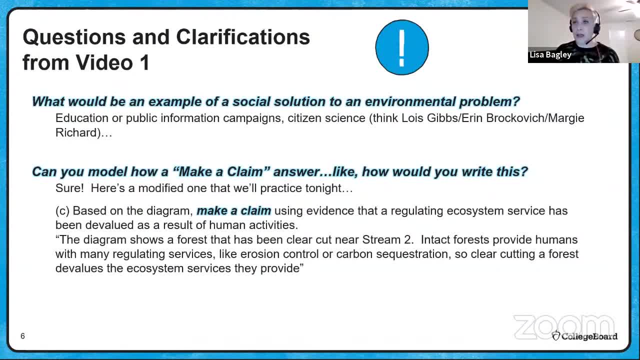 to do. several make a claims tonight, So here's a modified one. you know that I took from today's practice, Based on the diagram which you'll see later. make a claim using evidence that a regulating ecosystem service has been devalued as a result of human activities. Okay, So you've got. 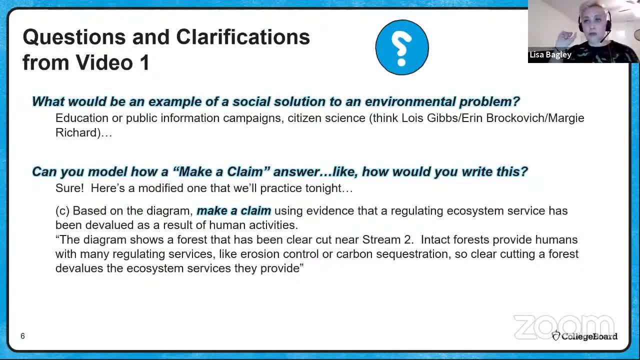 to make a claim you've got to use evidence from the diagram and you've got to specifically regulate the ecosystem services- Three things you've got to hit here. The diagram shows a forest that has been clear cut. near stream, two Intact forests provide humans with many regulating 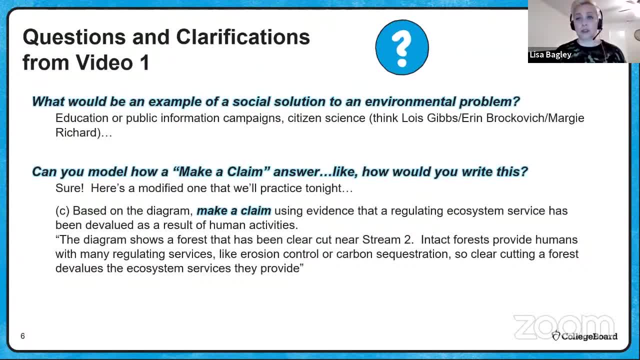 surfaces like erosion control and carbon sequestration. So clear cutting a forest devalues the ecosystem services they provide. I'm telling you that I saw in the diagram that there is a forest that's been clear cut right, And I know that intact forests provide ecosystem services. 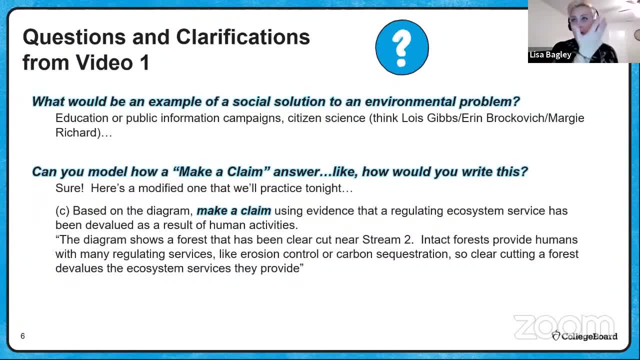 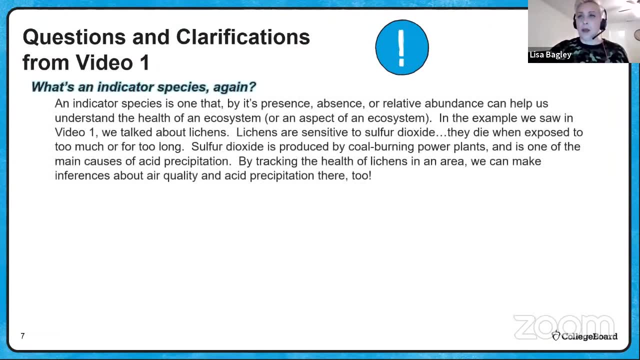 and I gave an example of that And I'm telling how the clear cutting would devalue those ecosystem services. That hits all three of those. Okay, So that's how it would look like in narrative format rather than rubric format. All right, Hey, what's an indicator? species again. All right, An indicator. 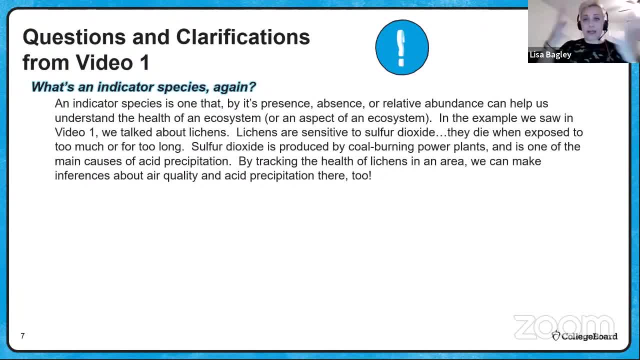 species is one that, by its presence, by its absence or by its relative abundance, can help understand the health of an ecosystem or the health of an aspect of an ecosystem. We did an example of this in video, one where we talked about lichens. Lichens are sensitive to sulfur. 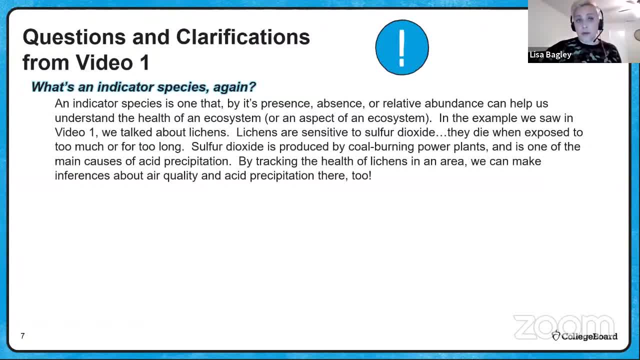 dioxide. They die when they're exposed to too much of it or exposed for it for too long. Sulfur dioxide is produced by coal burning power plants, and it's one of the main causes of acidic precipitation. By tracking the health of lichens in an area, we can also make inferences about air. 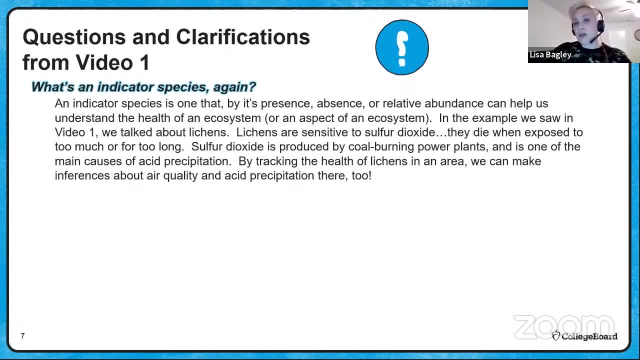 quality and acidic precipitation There. So this indicator species is telling us by its presence, absence or relative abundance, what's going on with air quality in an area. That's what an indicator species is. What's RLF? RLF is replacement level fertility. It refers to the number of children- women- in a population must have to sustain population levels. It's about two in developed nations a little more about 2.1.. But it's higher in developed nations, a little more about 2.1.. Like Niger, is around 7 for RLF because Niger has a really high infant and child mortality rate. So women have to have more children in order to offset the children that are dying before age five Are all generalists are selected. So, in reality, most species in the real world fall somewhere between R and 5.. So, in reality, R and 5 are down into the flow of our life. 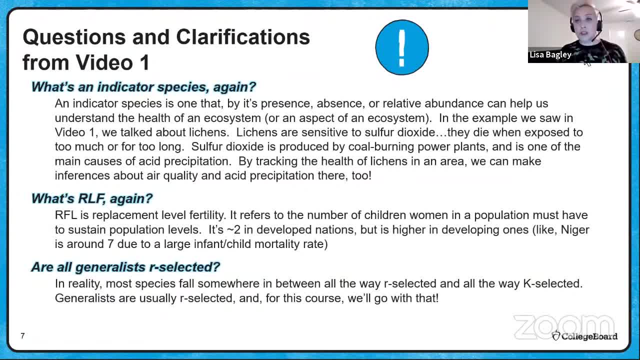 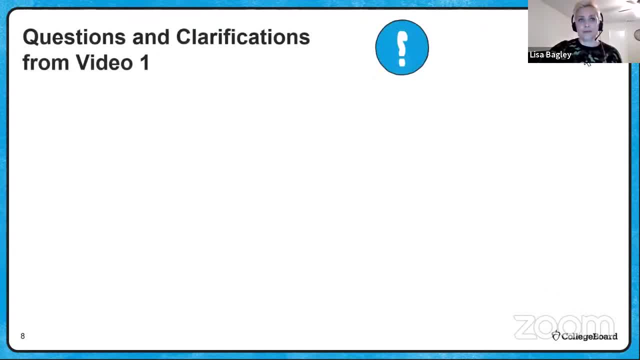 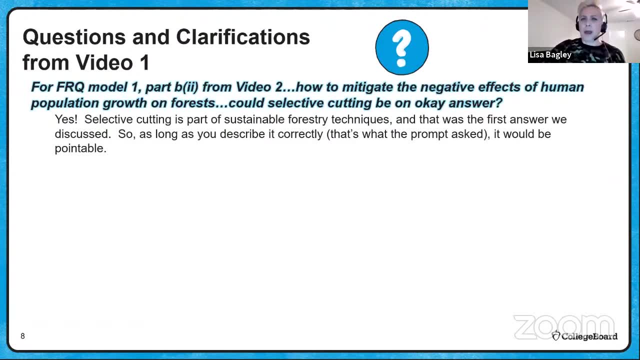 the way. K selected Generalists are usually closer to R selected and for this course we're going to go along with that kind of rule of thumb. All right, here's a specific one For free response, model one from video two. and just to refresh you how to mitigate the negative effects of human 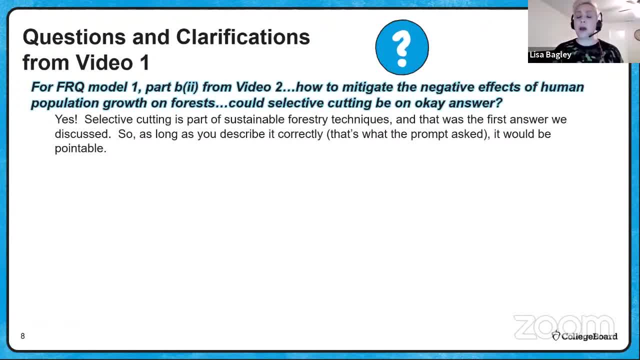 population growth on forests. Could selective cutting be an appropriate or okay answer? Thank you for asking very specific and I love it. The answer to that is yes, Selective cutting is actually part of sustainable forestry techniques, and that was the first answer discussed. So 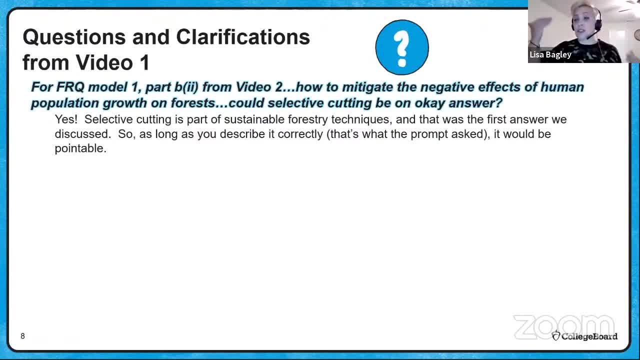 sometimes the rubric shortcuts this stuff. So if you mentioned a specific sustainable forestry technique and you described it correctly because the prompt asks you to describe it, then yes, it would have been pointable. You could have said sustainable forestry techniques or mentioned a. 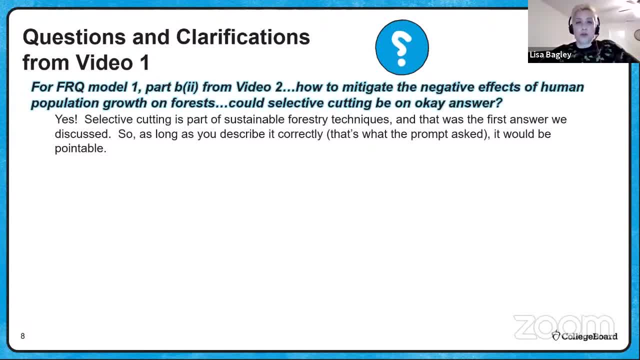 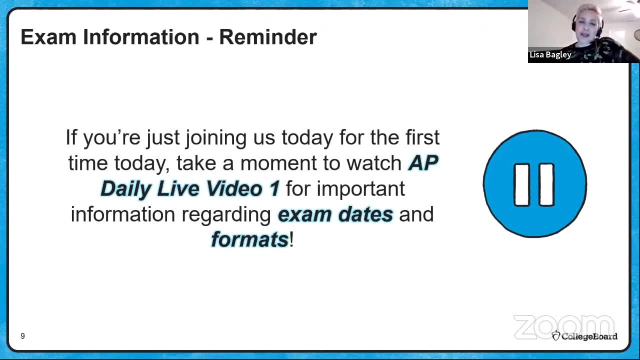 specific sustainable forestry technique. So, yes, it would have been pointable. Yes, perfect, wonderful, And I am proud of you because y'all's brains are getting so strong, Yay, All right, just some exam information reminders. So if you're joining us for the first time today, 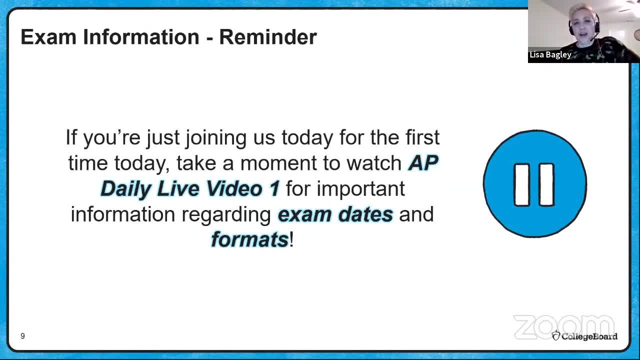 please, please, please, take a moment to watch AP Daily Live video one for important information regarding exam dates and exam formats. This is really important stuff and I want you guys to be prepared for whatever type of exam you're going to be taking. So, if you're going to be, 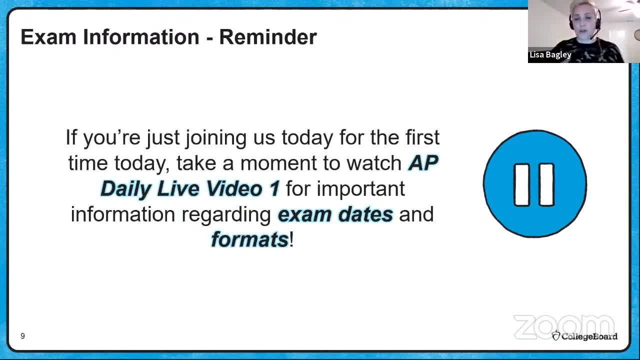 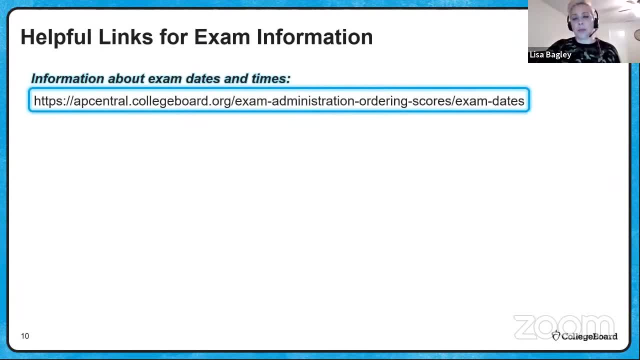 taking so that you can launch off wonderfully. All right, and, as always, I'm going to provide you with the helpful links for exam information. if this is your first time here, If you need information about general exam dates and times, there's your URL. If you need information, 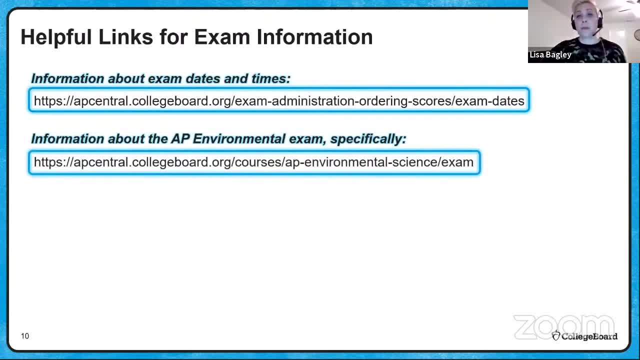 specifically about the AP environmental exam. there's your URL. If you are taking the digital exam and you're not taking the digital exam, then you're not taking the digital exam. So if you're not sure what to expect, there's your digital testing guide right there. Now, some of that is. 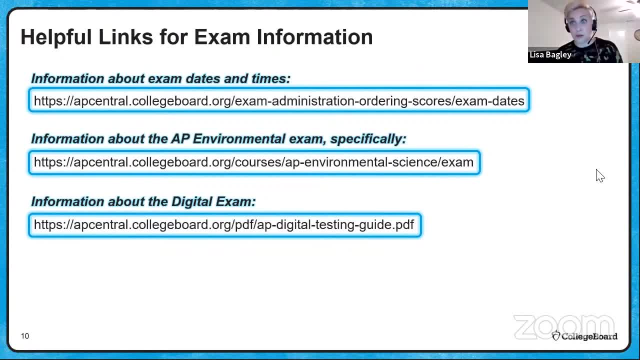 you know, with student-friendly, and some of that pertains to people that aren't students, So take that with a little bit of grain of salt there. And then the preview of the digital exam, including how to get your device ready, and the practice app is available at this app. I'm also going to go. 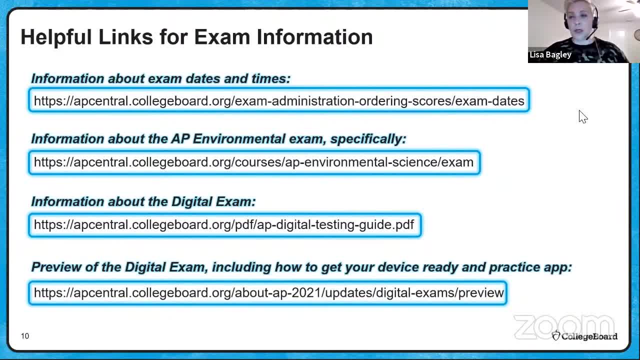 ahead and mention there is a YouTube video by the College Board that is giving that will give you information about the digital exam. So if you're not sure what to expect, there's your digital testing guide right there. So if you're not sure what to expect, there's your digital exam and how to get. 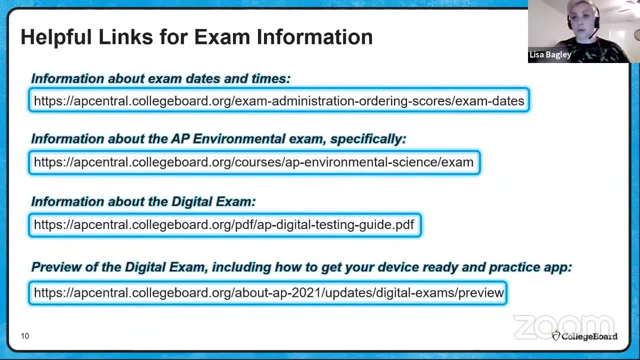 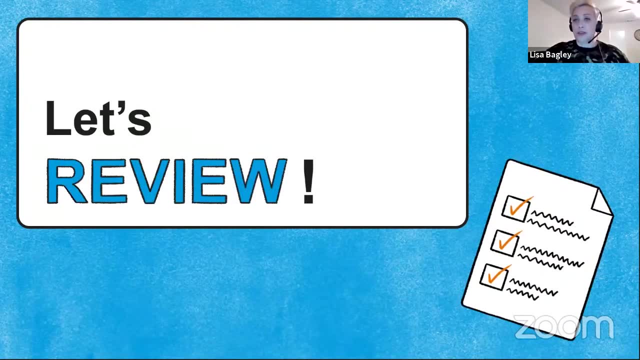 yourself ready. You can actually just search it up. It's right there in the channel for the College Board. So give it a try, Take a look, Get all your stuff that you need to get All right. So let's do some content review for Earth Systems, And I know like this is. sometimes kids are like what the 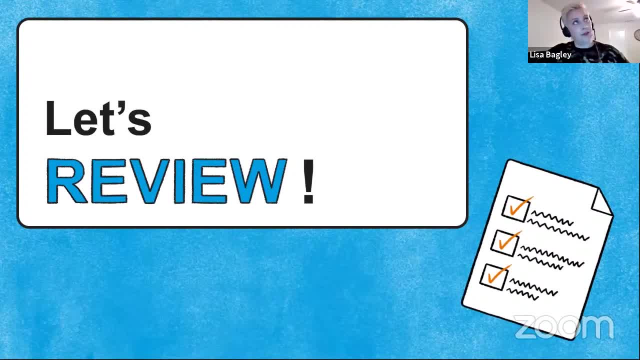 what Coriolis effect, huh. What Thermothelial circulation? huh. But trust me, this guy was going to be a geologist. He's going to be a geologist, He's going to be a geologist. He's going to be a. 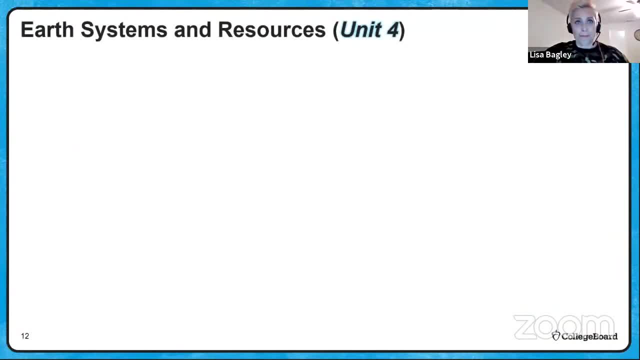 geologist, So you're in good hands, Let's get started, All right. Plate tectonics. Plate tectonics is the theory explaining the movement of Earth's rigid lithospheric plates That's the result of convection processes. convection processes in the underlying partially molten mantle right So the 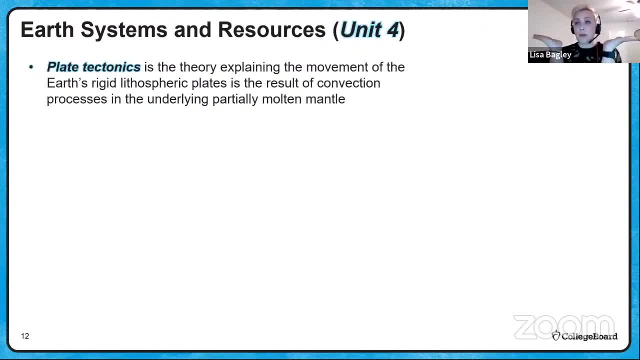 plates are moving because there's convection that's spreading them apart or bringing them together, due to the results of the earth's rigid lithospheric plates. So the plates are moving because there's convection that's spreading them apart or bringing them together, due to the results of 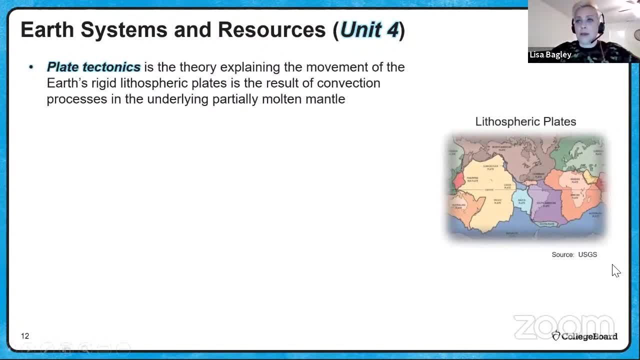 the molten mantle. This is a little map of our lithospheric plates here on Earth. These lithospheric plates have distinctive features where they either come together, which is converging, pull apart, which is diverging, or push against each other. I want to talk about each of those Convergent. 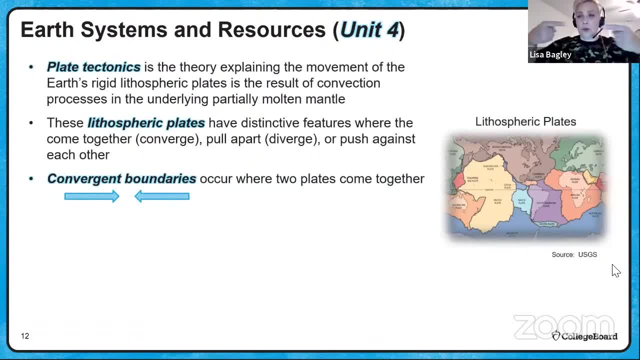 boundaries occur where two plates come together. Two plates come together. Features of convergent boundaries depend on the amount of heat that's in the plate. So if you have a plate that's converging, it's converging on the types of crusts that are converging- oceanic or continental. 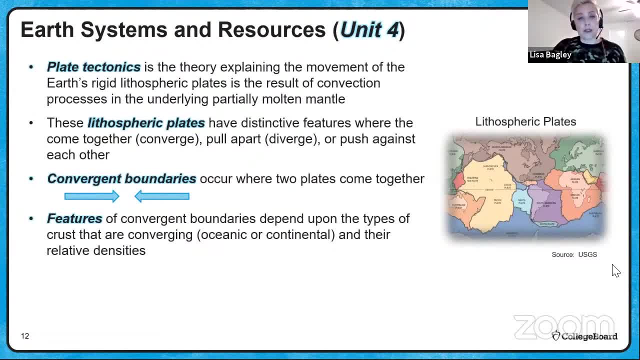 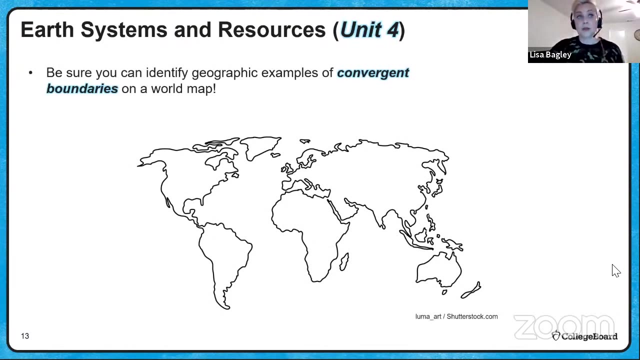 oceanic are under the oceans and continental are under the continents and their relative densities. Convergent boundaries create mountains, island arcs, earthquakes and volcanoes, And you need to be able to identify those on a map. So be sure you can identify the geographic examples of convergent boundaries on a world map. 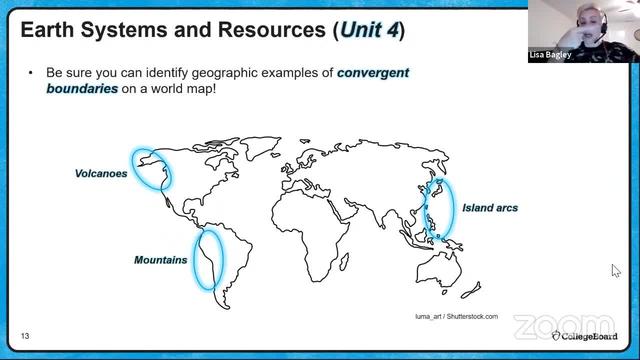 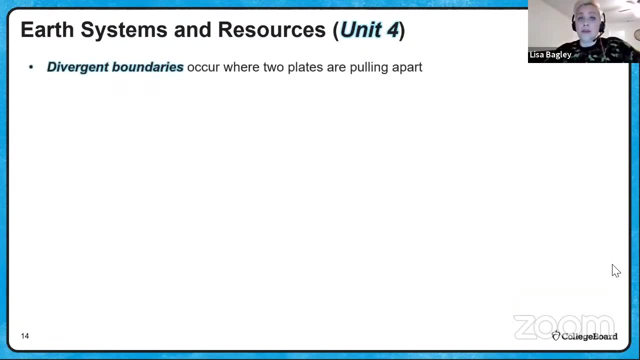 like island arcs, volcanoes and mountains. Island arcs there in the Pacific, Japan down to Indonesia. volcanoes in the Pacific Northwest and the Andes. Divergent boundaries occur where two plates are pulling apart. Pulling apart Divergent boundaries can result in convergent boundaries on a world map. like island arcs, volcanoes and mountains, Island arcs there in the Pacific, Japan down to Indonesia, volcanoes in the Pacific Northwest and the Andes, Divergent boundaries occur where two plates are pulling apart. Pulling apart Divergent boundaries can result in 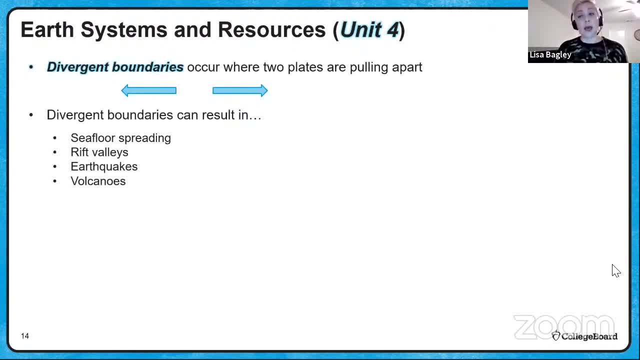 sea floor, spreading rift valleys and also earthquakes and volcanoes. Transform boundaries occur where two plates are trying to slide past each other, usually horizontally, We're at an angle, but they're not diverging and they're not converging. They're trying to kind of slide past each other And they're under pressure. 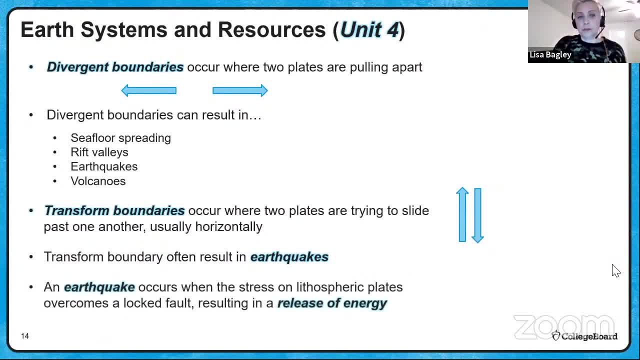 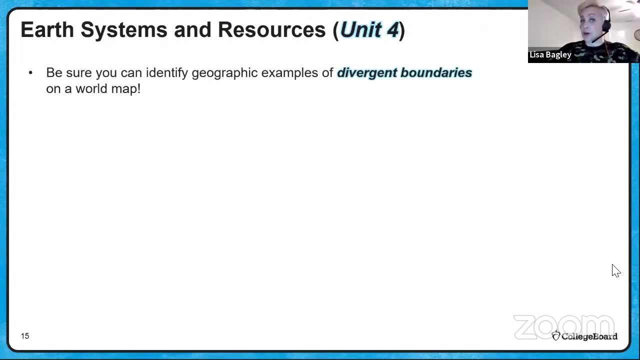 Transform boundaries often result in earthquakes. An earthquake occurs when two plates are pulling apart. An earthquake occurs when the stress on these lithospheric plates overcomes a fault that is locked, resulting in a slip and a release of energy. Be sure you can identify geographic examples of divergent boundaries on a world map like this. 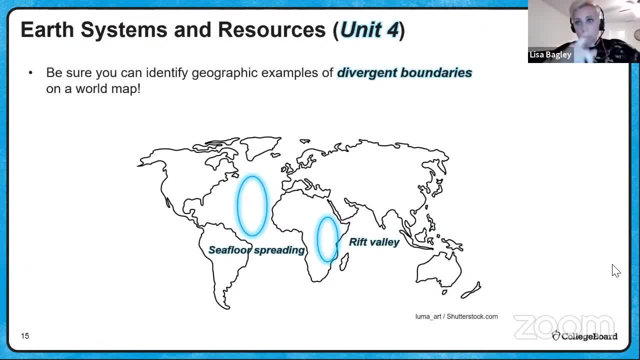 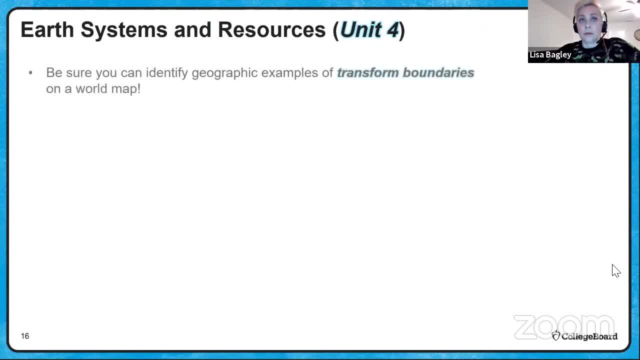 Sea floor spreading in the mid-Atlantic rift. Yes, I know that that circle looks like it's circling nothing, but that's the mid-Atlantic rift And the rift valley in East Africa, And be sure that you can identify geographic examples of transform boundaries on a world map. 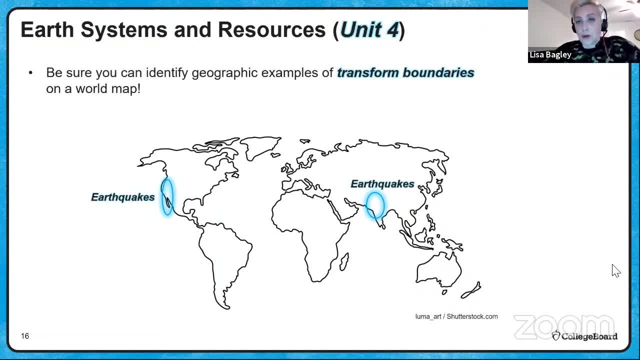 Earthquakes occur. That's the San Andreas Fault, And earthquakes are occurring there in the Himalayas as well. Now, obviously, there's a lot more examples geographically that we could give for each one of these faults, So these aren't the only ones that you could see. I'm just giving a couple of overview examples. 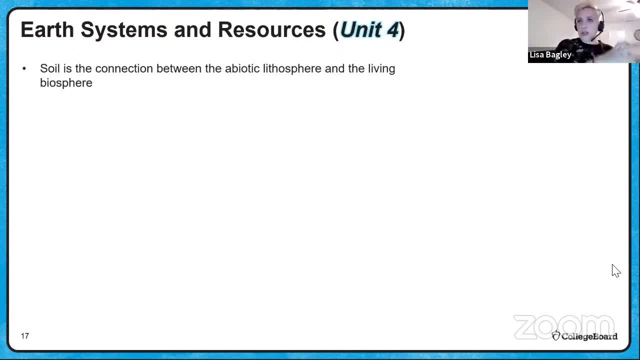 All right, let's talk about soil. So it's a jump from lithospheric plates to soil, But soil is really the connection between these abiotic lithospheric plates and the living biosphere that we're going to study. Soil is formed when parent material is weathered, transported and deposited. 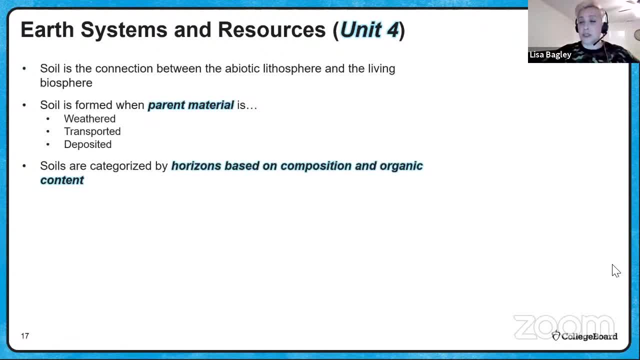 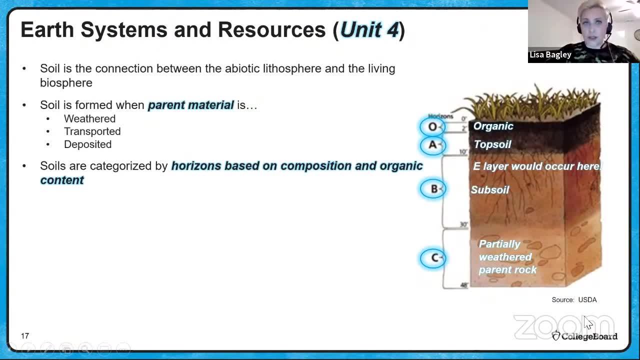 Soils are categorized by horizons based on composition and organic content. Yay, soil horizons. So this is like a cross-section of a soil horizon. We've got our organic layer, our O horizon, at the top. top soil, which is our A horizon, comes next. 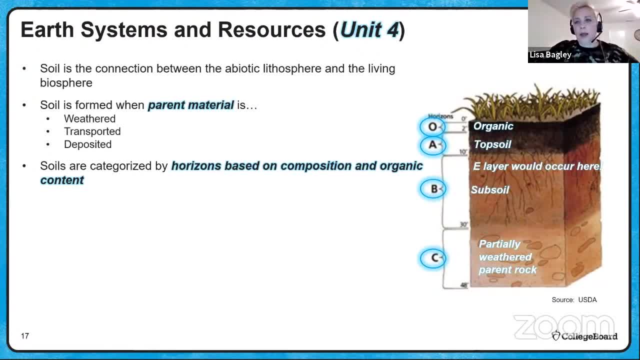 I'm going to skip the E for right now. B is our subsoil and C is the partially weathered parent rock. Not all soils have an E layer. It depends on the climate and it also depends on the age of the soil. 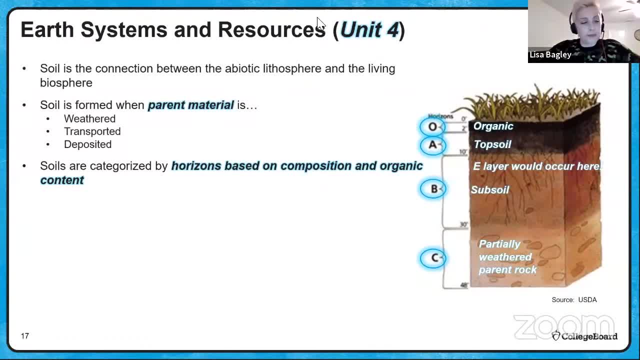 But you might actually see an E layer on the exam as well. Soils are a cross-section of a soil horizon. Soils are, of course, an important natural resource that must be protected And there's a lot of questions that pertain to soil health, soil erosion, because soil really is that link between biotic and abiotic conditions. 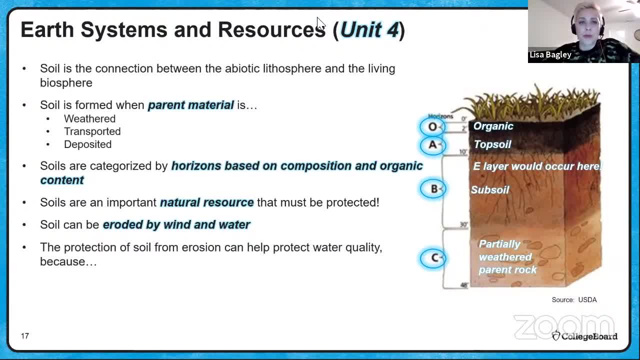 Soil can be eroded by wind and water, And the protection of soil from erosion can actually help protect water quality, because soil helps to filter and clean water, ecosystem service And soil erosion into bodies of water can create turbidity. It can also reduce the soil moisture. 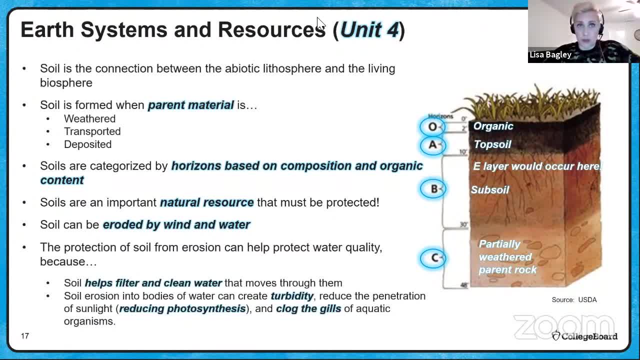 It can also reduce the penetration of sunlight, which reduces photosynthesis, which of course is the basis of the trophic structure in an ecosystem, And it can clog the gills of aquatic organisms. Soil is pretty darn important in AP environmental science. 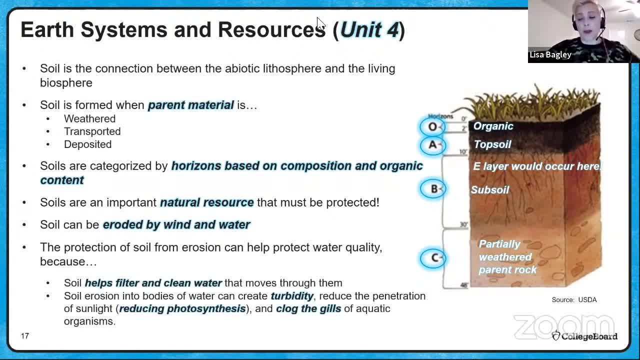 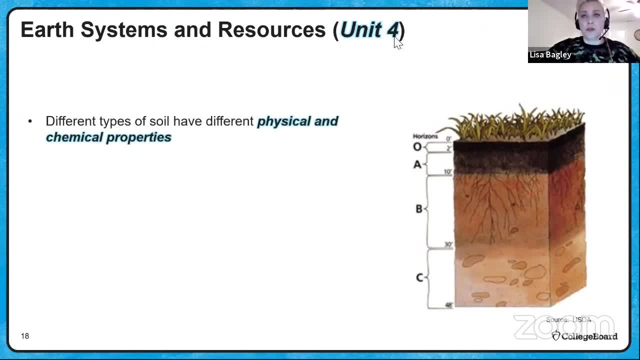 So you'd do a good favor to yourself by going back and reviewing your soil stuff. All right, Different types of soil have different physical and chemical properties. Water holding capacity is the total amount of soil. Water holding capacity is the total amount of soil. 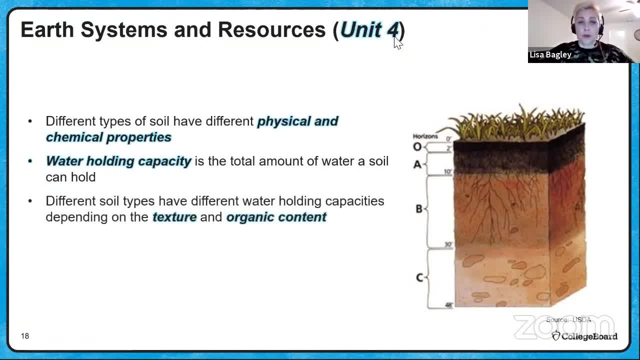 water that a soil can hold. Different soil types have different water holding capacities depending on their texture, their percentage of sand, silt and clay- and we're going to get to that in a minute- and their organic content. The ability of a soil to retain water contributes. 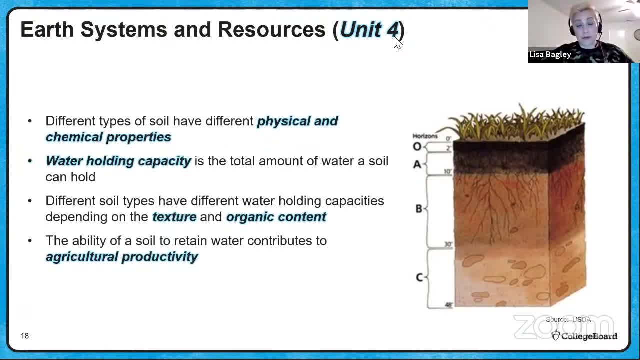 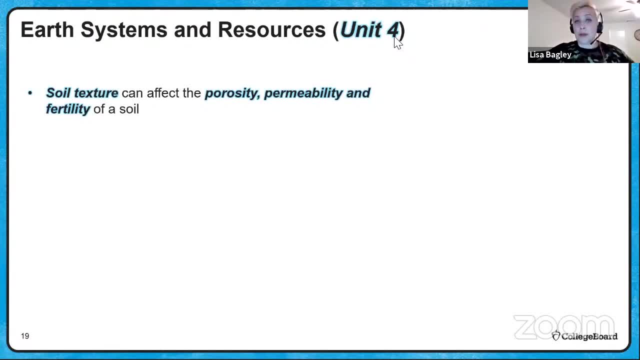 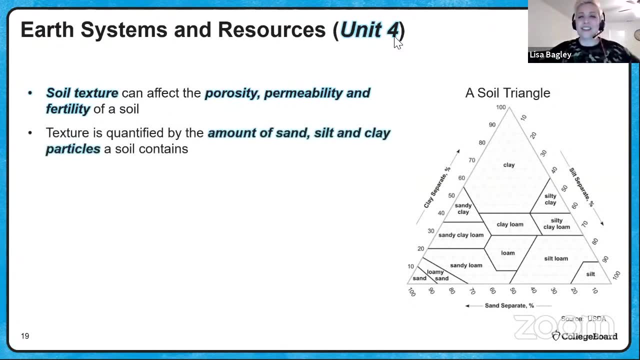 of course, to agricultural productivity, and we'll talk more about that in Unit 5 tomorrow. Soil texture can affect porosity, permeability and the fertility of a soil. Hey, it's a soil triangle. Texture is quantified by the amount of sand down there at the bottom silt right-hand. 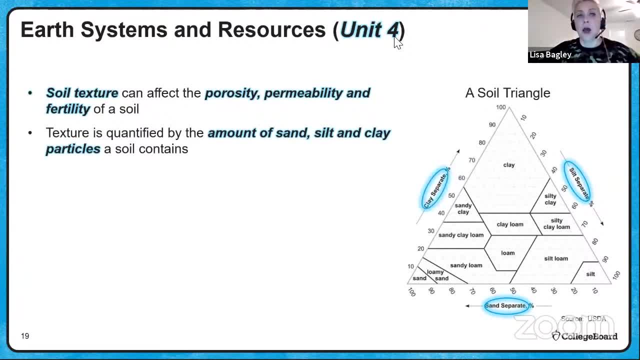 side and clay on the left-hand side, particles that a soil contains. You do need to know how to read a soil triangle. This is in our Unit 4.. Videos will take you through it, so please, please, please, if this is the first time you've. 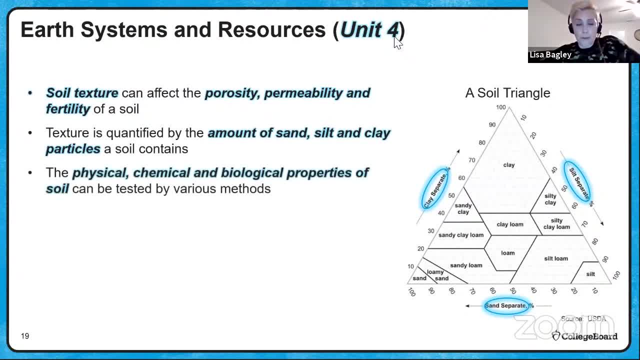 seen a soil triangle and your mind is blown. go back and look. The physical, chemical and biological properties of soil can be tested by various methods. Hint, hint, experimental design. Soil tests can help determine agricultural irrigation needs and fertilizer requirements. 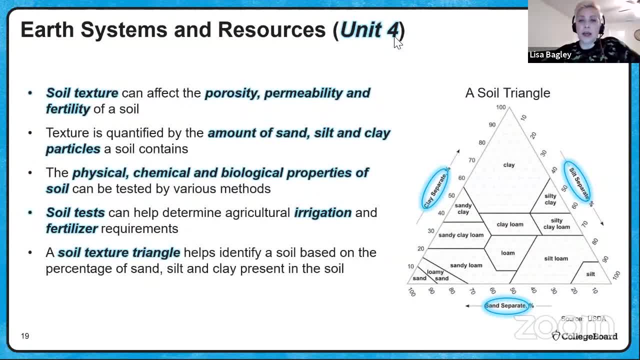 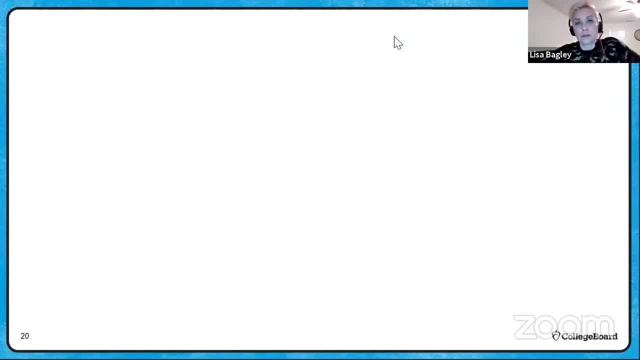 There's your soil texture triangle, and it can help you identify the type of soil based on its texture or its percentage of sand, silt and clay. All right, let's move from soil to the atmosphere. Earth's atmosphere is made of about 78% nitrogen. 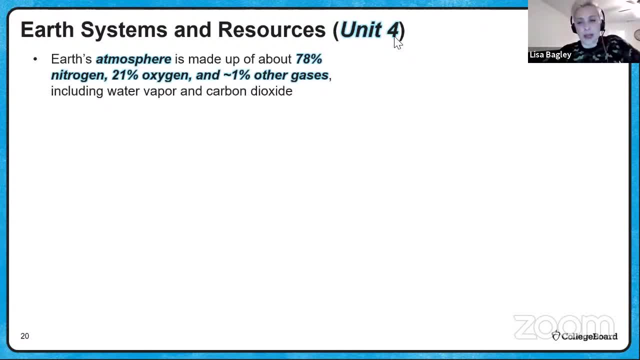 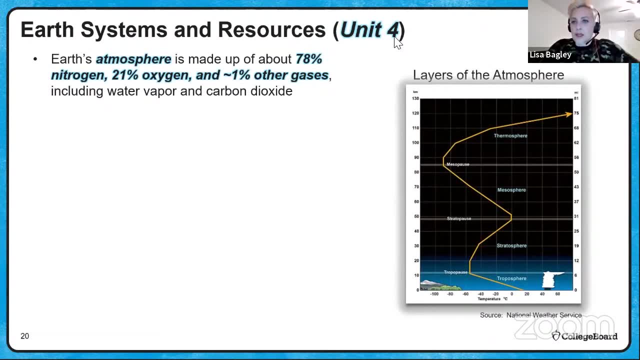 21% oxygen and about 1% other gases, including carbon dioxide and water vapor. This is a little side view of the temperature gradients of the atmosphere. The layers of the atmosphere are based on temperature gradients- The troposphere. let's talk about the troposphere. If you look at the diagram there. 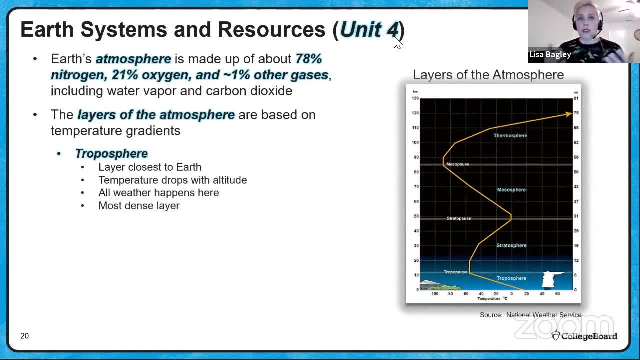 the troposphere is the layer that is closest to the Earth. The temperature in the troposphere drops with altitude, meaning it gets colder as we go higher. All weather happens in the troposphere. So if we're talking about weather, we're talking about the troposphere. So your 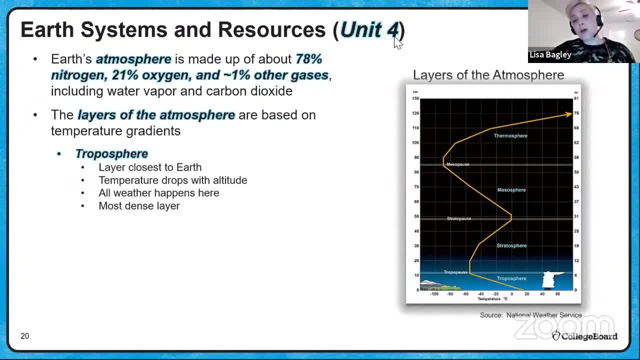 water vapor, your clouds, all the weather is happening in the troposphere. It is also your most dense atmospheric layer, because the most dense atmospheric layer is the atmosphere, So it's the most. particles exist here. The particles of air exist here. The stratosphere is above the 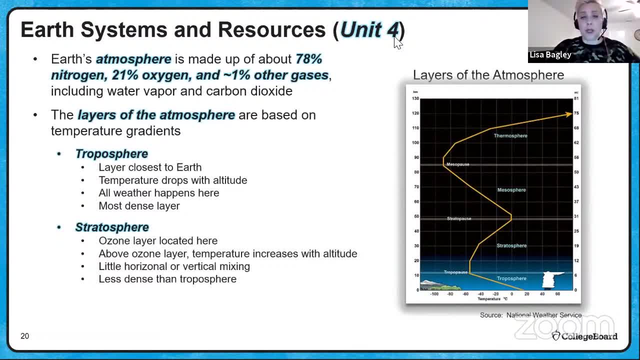 troposphere. This is where the ozone layer is located And you can kind of see this in the diagram. That little straight up and down in the lower stratosphere is where the ozone layer is. But above the ozone layer the temperature of the stratosphere actually increases with altitude And 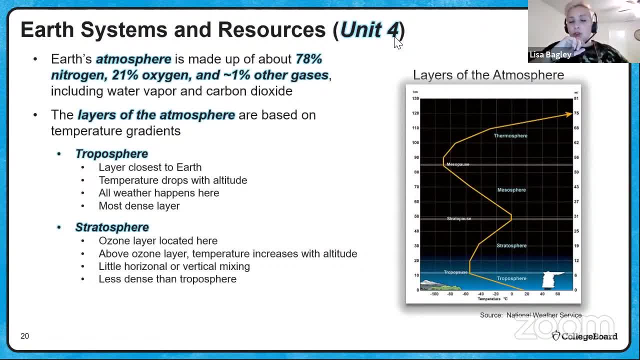 you can see that that zigzags back from the troposphere. There is very little horizontal or vertical mixing of the particles, So what goes up there stays up there, And that has some implications when it comes to chlorofluorocarbons. 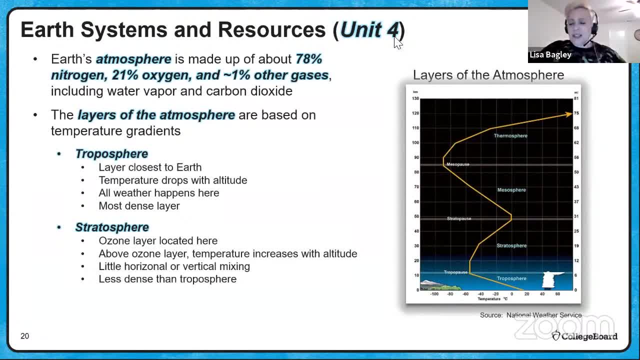 and bromated fluorocarbons and all that good stuff. It is less dense in the troposphere. There is less atmospheric particles up there And we got the mesosphere. And you can see that the mesosphere actually also gets colder with altitude. As we go up it gets colder. We've got the thermosphere. 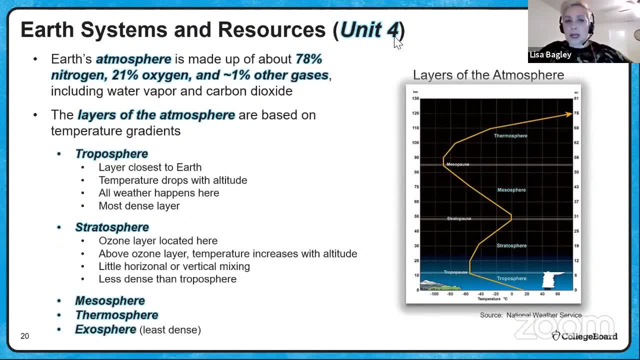 And finally the axisphere. The axisphere is our least dense. The troposphere and the stratosphere are going to be your biggies for environmental science, And you do need to know what happens there. Global wind patterns are the result of differential 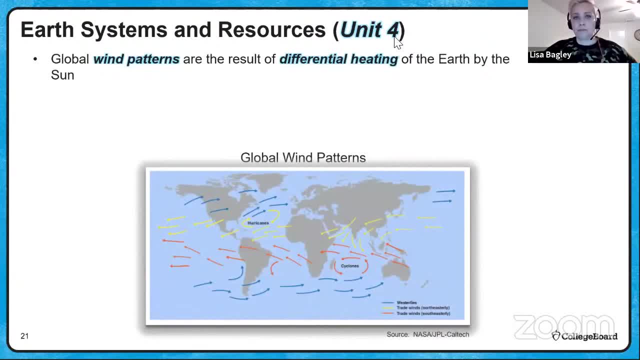 heating of the Earth's surface by the sun Yay global wind patterns. The most intense solar radiation arrives at the equator. This causes surface heating, which leads to density differences in the air. And these density differences, which is what we call the atmospheric circulation, lead to our tricellular model of atmospheric. 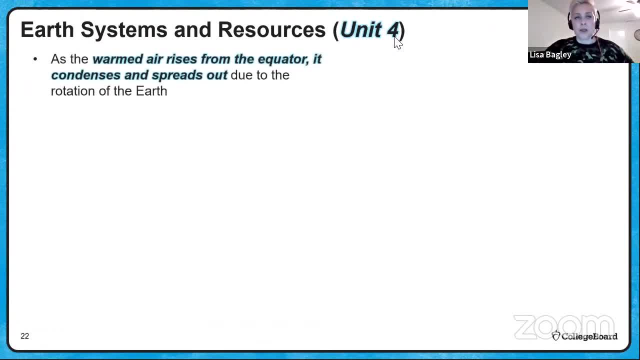 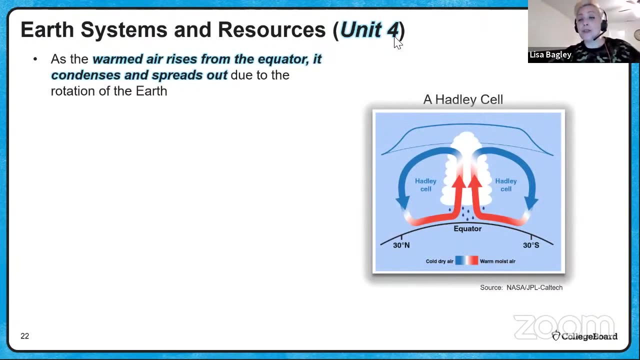 circulation. So let's talk a little bit about that tricellular model. So we have this direct incoming solar radiation at the equator And this warm air rises at the equator And it condenses and spreads out And this is due to the rotation of the Earth. Take a look at this picture right here. This is the 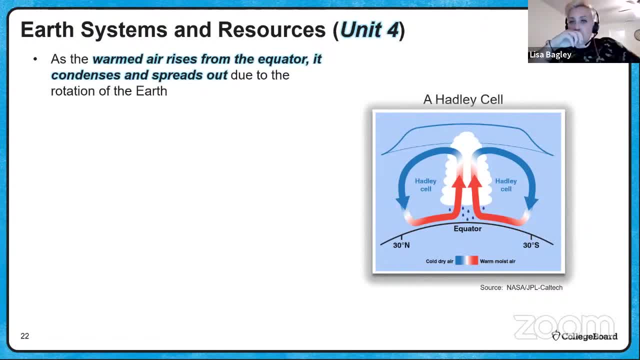 diagram of a Hadley cell. So you can see, there at the equator you've got really intense solar radiation. That warm surface air rises And then it spreads out to the north and to the south, away from the center line of the equator. The precipitation from this condensation falls. 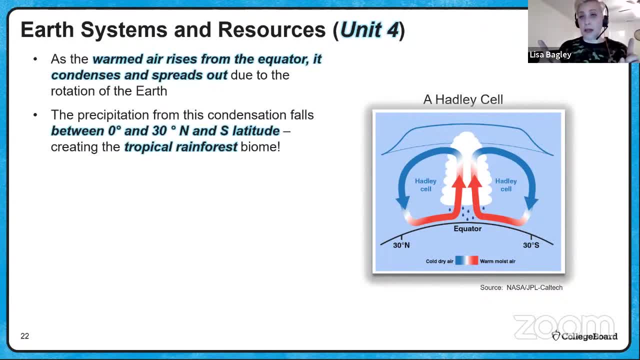 between zero and 30 degrees north and south latitude. That's our latitude for our Hadley cell right And that creates a tropical rainforest biome in that zero to 30 degrees north and south latitude And you can see there that the red obviously indicates warm, moist air And the 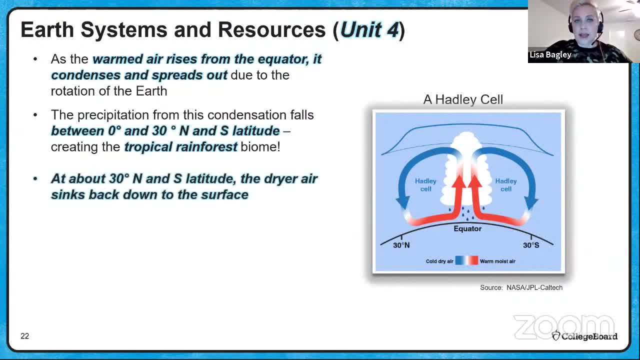 blue indicates cool, dry air And the red obviously indicates warm, moist air And the blue indicates cool, dry air. So at 30 degrees north and south latitude that cooler, drier air comes back down to the surface And that has implications for climate there. At 30 degrees north and south, 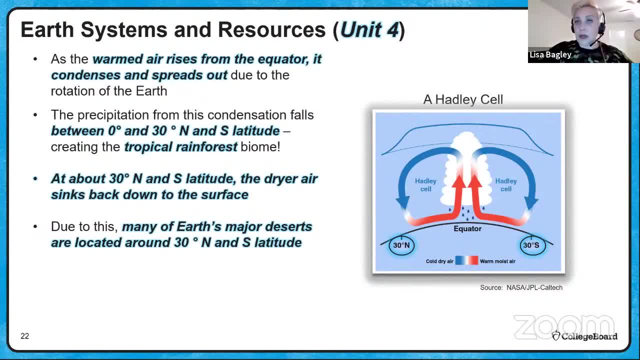 latitude we find many of Earth's major deserts, And that is because the cooler, drier air from the Hadley cell descends at those latitudes. This pattern of heating rising, condensing, precipitation and descent also occurs at our mid-latitudes- Those are our ferrule cells- And at the poles, which are the 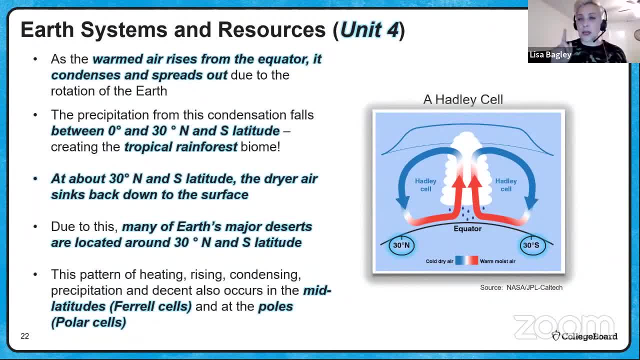 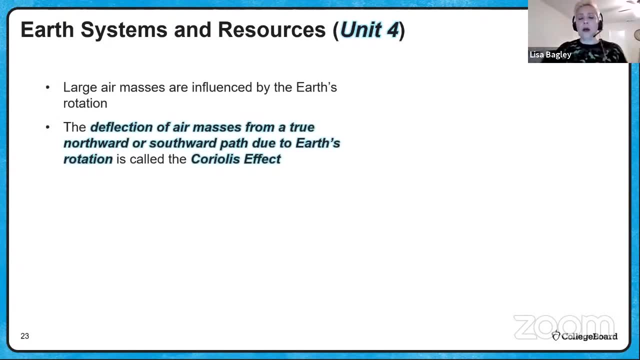 polar cells. So just a quick reminder if you can't remember which one's which. here's a little mnemonic. The Hadley happens where it's hot. at the equator Hadley is hot, All right. Large air masses are influenced by Earth's rotation. It's spinning on its axis, The deflection. 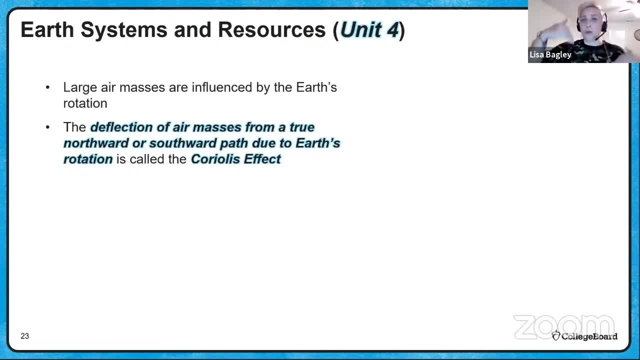 of air masses from a true northward or true southward path due to this rotation, is called the Coriolis effect. Objects, any object, including air masses, are deflected to the right in the northern hemisphere and to the left in the southern hemisphere due to the Coriolis effect. 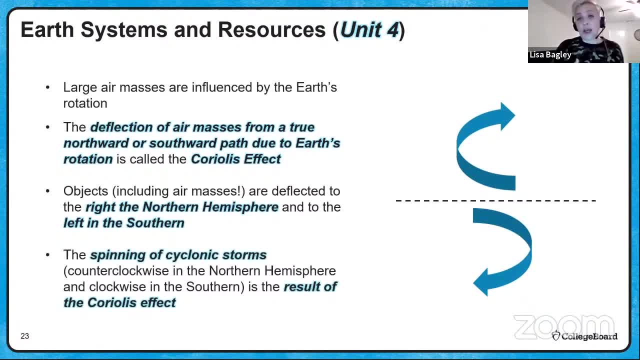 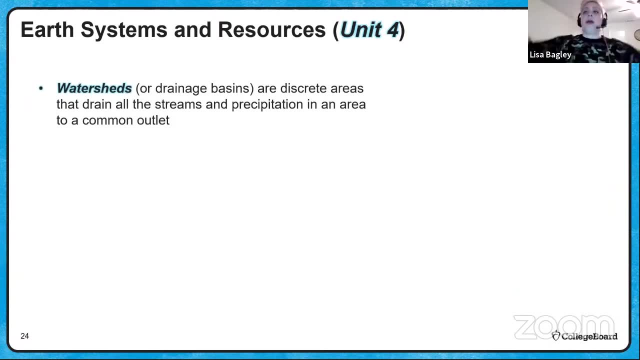 the spinning of the Earth on its axis. The spinning of cyclonic storms, which is counterclockwise in the northern hemisphere and clockwise in the southern hemisphere, is called the Coriolis effect. All right, We're moving from the atmosphere back down Watersheds or drainage basins. 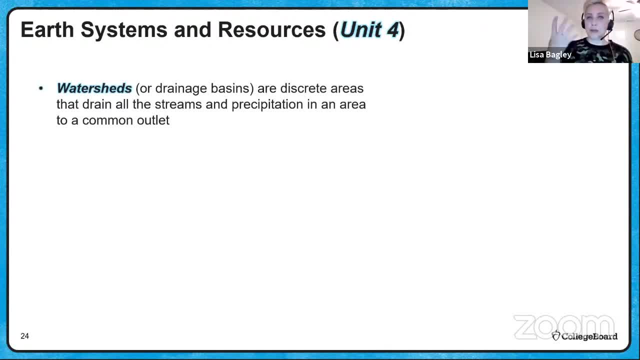 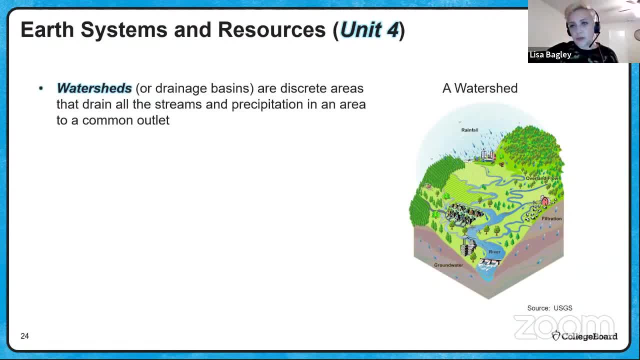 stuff going on here. There's a river. There's got groundwater infiltration, There's some farms, There's forests. There's a lot going on here. There's a town. Characteristics of a given watershed include its area, its length, the slope. Does it have a high slope or a low slope? 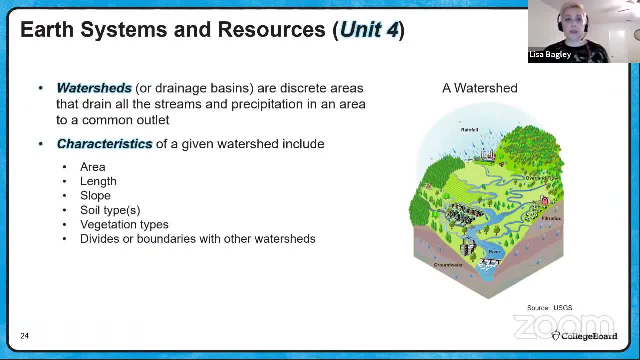 The soil types that underlay it, vegetation types and divides or boundaries with other watersheds. Watersheds and water quality, of course, are affected by human activity, And we're going to actually model this with a free response question today. 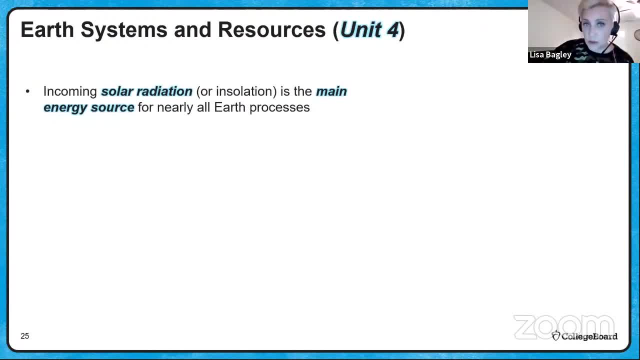 Incoming solar radiation, which is also called insolation, is the not insulation like in your attic, but insolation. incoming solar radiation is the main energy source for nearly all Earth processes. The intensity of insulation varies by season and by latitude because these factors 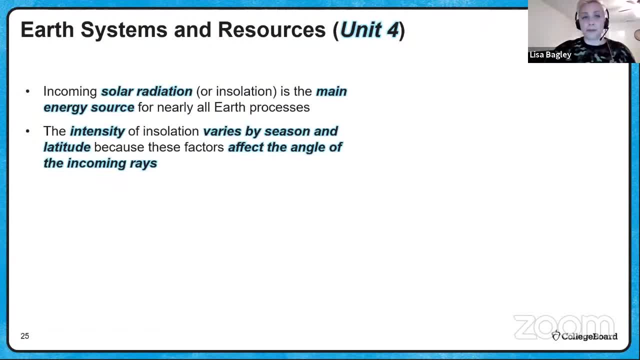 affect the angle of the incoming rays. All right, So this is a little graphic, talking about the angle of incoming solar radiation. So let's pretend that the sun is a flashlight, right? And if you have a piece of paper and you shine your flashlight, 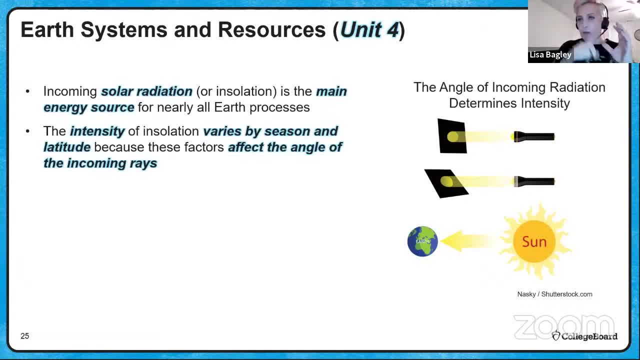 directly right, you get a nice round piece, a nice round beam of light there. But if you tilt your paper right, you're going to have an oblique angle there, And so the same amount of incoming solar radiation is going to have to spread out over a greater geographical area. So if you have a 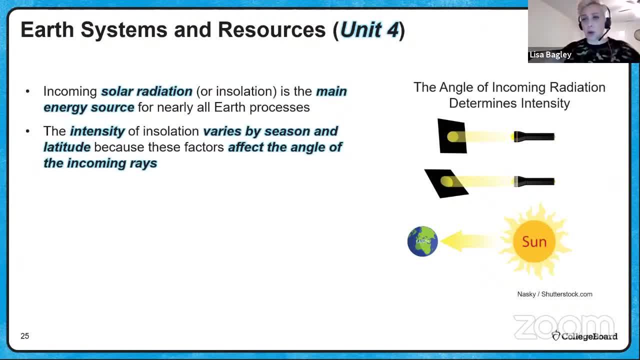 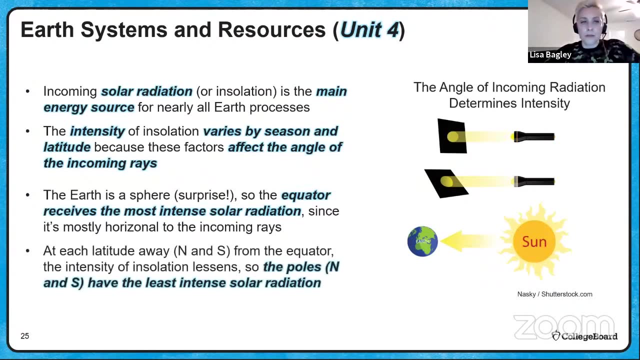 so, at any given area, your intensity will be lower. The Earth is a sphere. Surprise, it's a sphere. So the equator receives the most intense solar radiation, since it's mostly horizontal to the incoming rays. At each latitude away from the equator, both north and south, the intensity of 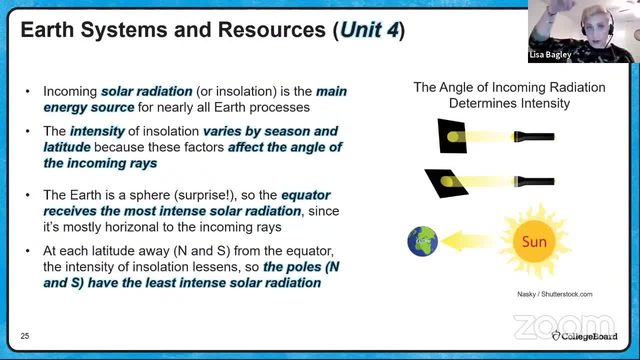 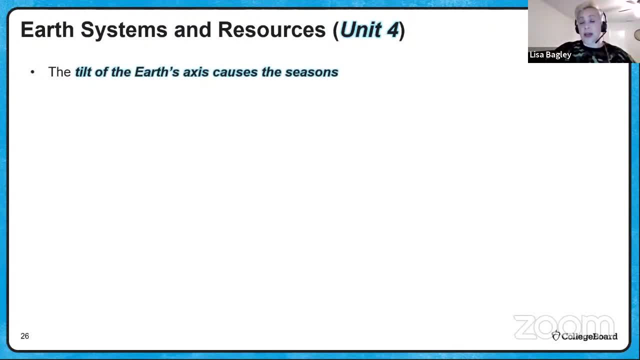 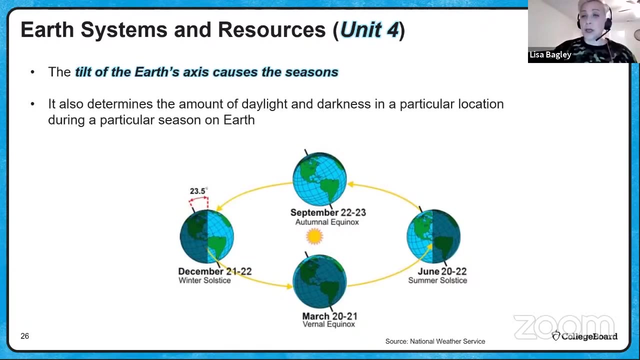 this insulation lessens, So the poles, north and south have the least intense solar radiation. The tilt of the Earth's axis causes the seasons There. she blows Tilt. It also determines the amount of daylight and darkness in a particular location during a particular season on Earth. 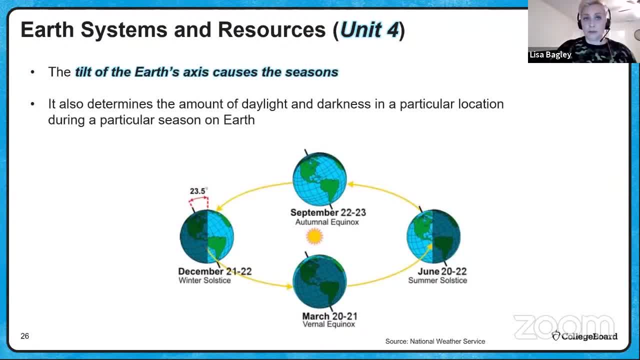 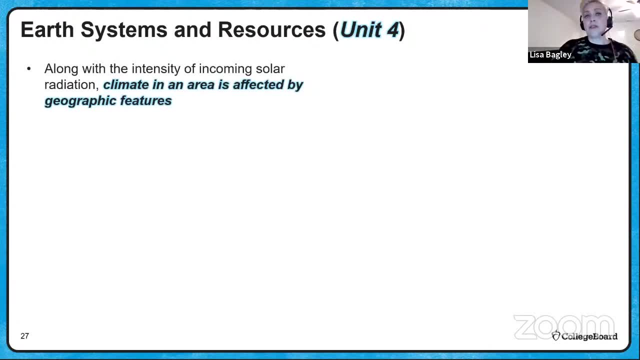 And again, we will practice this today. Along with the intensity of incoming solar radiation, climate in an area is affected, And these include mountains and proximity to large bodies of water. Normally, warm surface air rises and cools as it moves up into the troposphere, But we have a phenomenon called a thermal inversion. 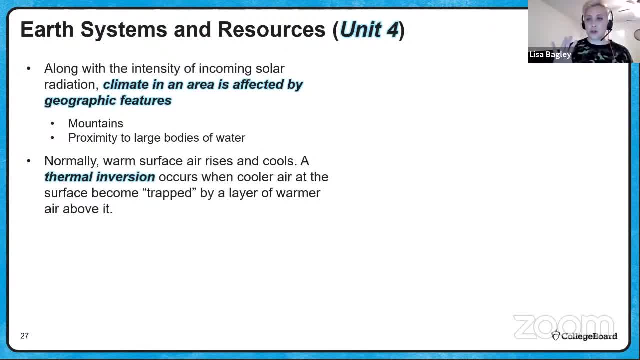 A thermal inversion occurs when cooler air at the surface becomes trapped by a layer of warmer air above it. Remember that this is all caused by density differences, and warmer air rises, And so that's going to stay on top of your more dense, cooler air. This is a problem, because thermal 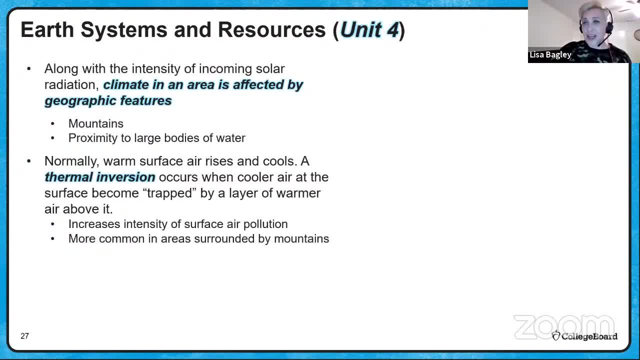 inversions increase the intensity of surface air pollution, It traps the ability of that air pollution to rise up into the troposphere and spread out, And thermal inversions are more common in areas that are surrounded by mountains. So, again, geographic features are going to influence. 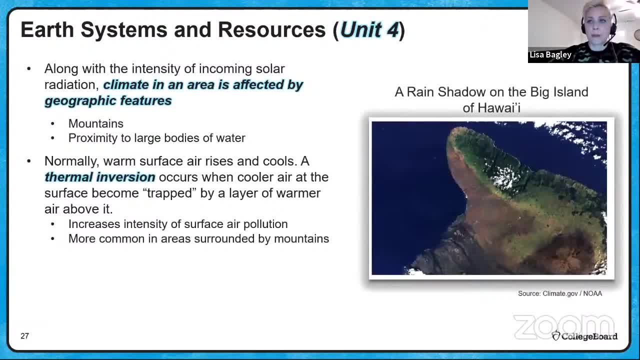 the intensity of your thermal inversions. Let's talk about rain shadows. A rain shadow is a rain shadow that is a dryer area of land adjacent to or in the shadow of a higher elevation. The higher elevation, like a mountain, blocks the precipitation from reaching this area And there's a picture That's the big island of Hawaii. 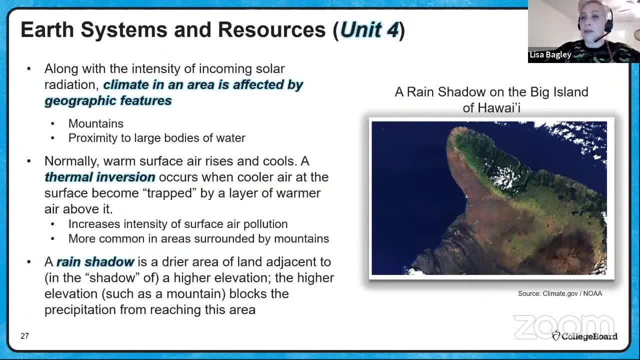 And you can see that one area is very green and lush and the other side is actually kind of brown and dry And that is your rain shadow side. So the precipitation is falling on one side and then all of the by the time the air gets to the downward slope. 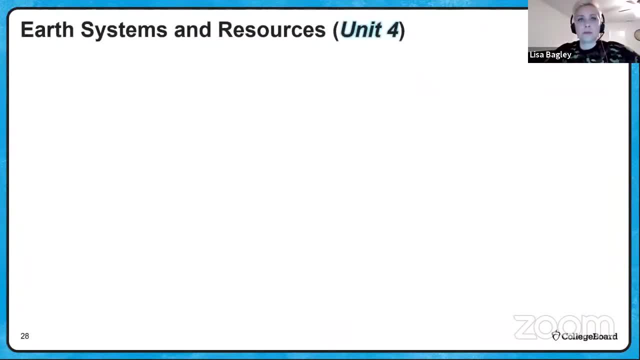 all of its moisture is gone. Ocean surface temperatures help to drive oceanic circulation patterns. Surface temperatures fluctuate, in part due to changes in the prevailing winds, which we talked about a few slides ago. So two things that you need to know are El Niño and La Niña conditions. 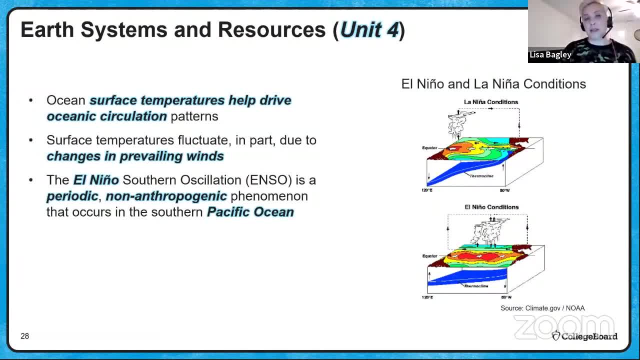 The El Niño Southern Oscillation, or ENSO, is a periodic, non-anthropological anthropogenic phenomenon. That means it's not created by man and it occurs in the Southern Pacific Ocean. So what we would call the normal conditions would be our La Niña conditions. 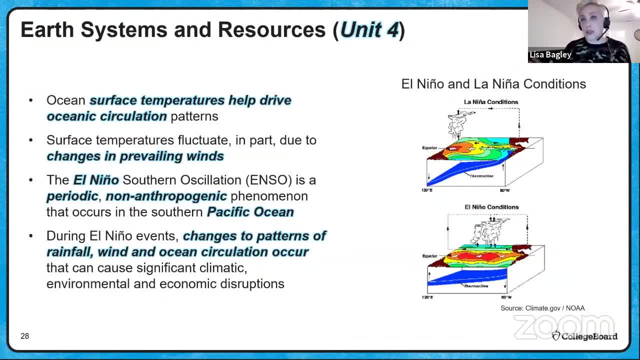 But I don't want to really classify as normal or abnormal because El Niño is just a periodic, naturally occurring event. However, it does cause disruptions. During El Niño events, changes to patterns of rainfall, wind and ocean circulation occur. 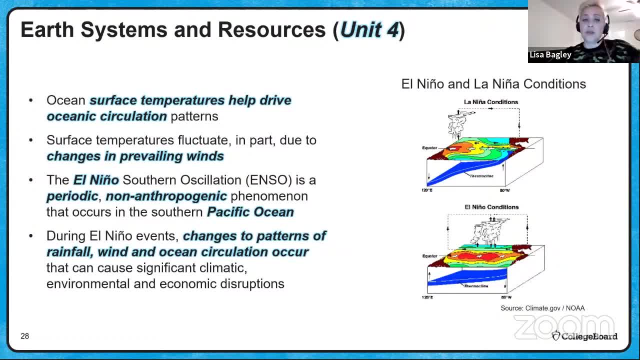 That can cause significant climatic, environmental and economic disruptions. So basically, what happens here is the prevailing winds coming over the Andes and through the plains of South America weaken, And when they do, they're not able to push this warmer surface water across the South Pacific over to Australia and the Indonesian area. 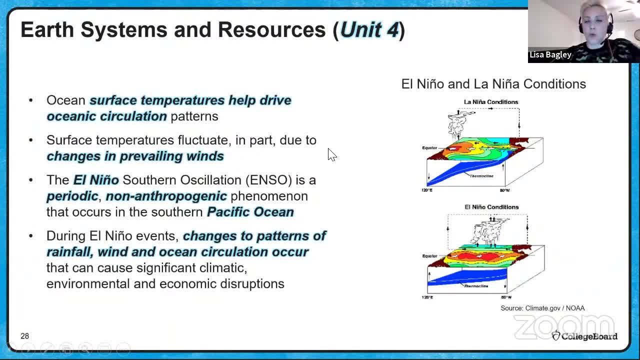 Normally we've got these strong surface winds that push our warm surface water across to the opposite side. So we've got our cold upwelling that comes from the deeper layers. We've got this thermocline, and our cold upwelling brings nutrient-rich waters to the coast of South America, which helps the fishing grounds there. 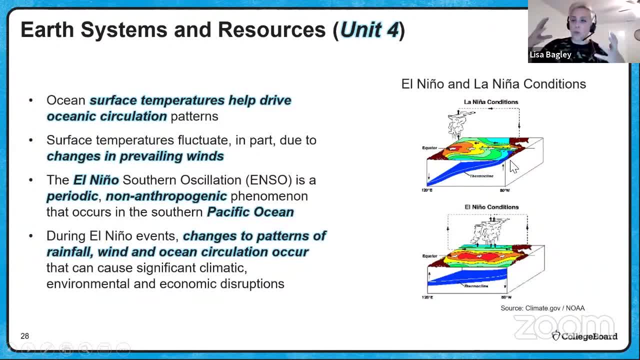 It also makes sure that that warm, moist air that's needed for precipitation across in Australia and the Indonesian area gets pushed over. that way keeps those conditions drier on the coast of South America. But when those prevailing winds weaken, then our thermocline declines. 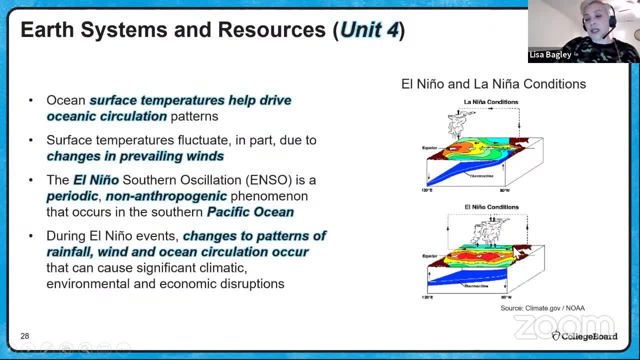 We don't have that upwelling and our warm, moist surface air gets trapped here over the coast of South America. We have wet conditions, things prone to mudslides there, And then we also have a lack of fishing because those cold, nutrient-rich waters don't come up on the coast. 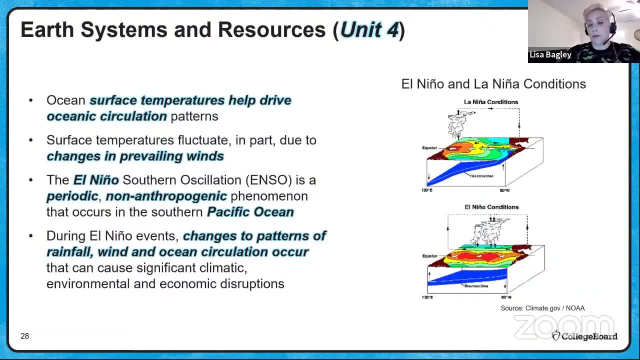 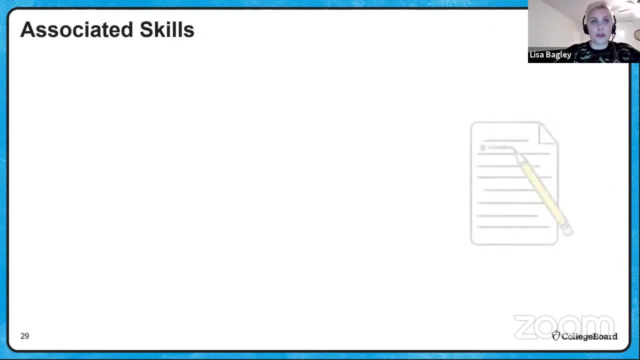 So you do need to know what happens for climatic, environmental and economic disruptions during an El Niño event. All right, so let's talk about skills associated with this unit. Remember that any skill can be tested in any unit, but there are certain units that lend themselves to certain skills. 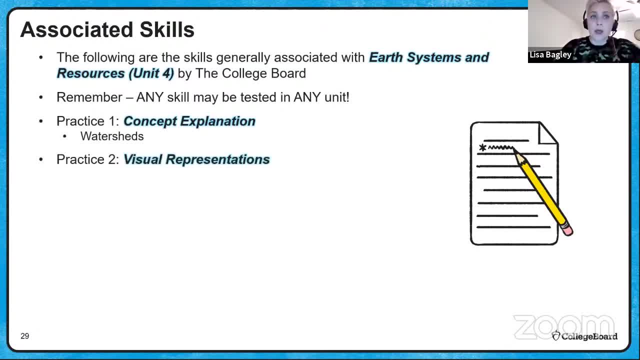 So practice one, concept explanation, watersheds. Practice two: there's a lot of practice two in unit four. I want to talk a lot about that: Plate tectonics, Earth's atmosphere, global wind patterns, solar radiation and the Earth's seasons, Earth's geography and climate. 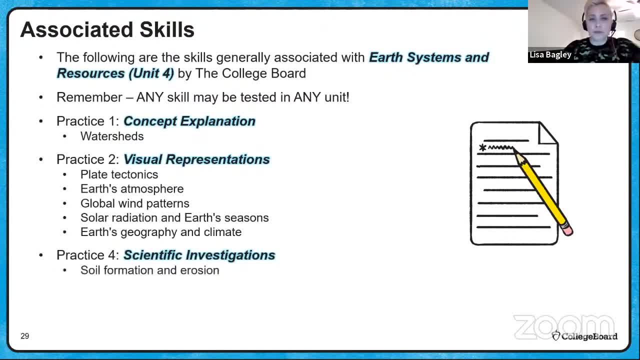 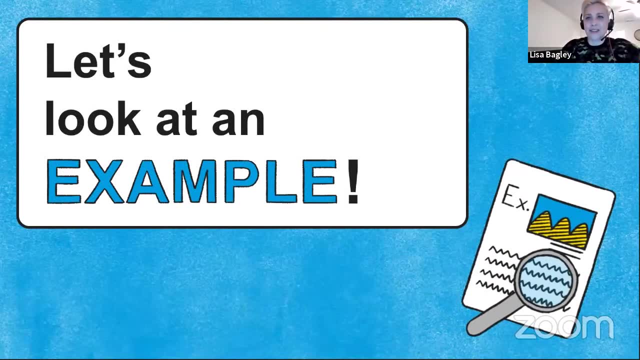 Practice, four scientific investigations: soil formation and erosion, soil composition and properties And finally, our environmental solutions, where we're providing solutions and justifying those. El Niño and La Niña. All right, let's take a look at our first example for today. 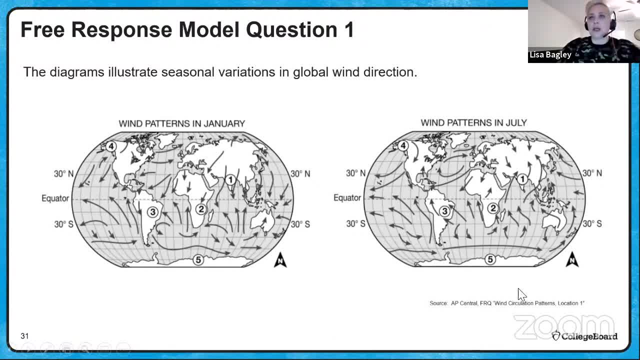 The diagrams below illustrate seasonal variations in global wind direction. So I'm going to start with this. This unit is visual model heavy and these visual models can be overwhelming when you first look at them. You look at this and you're like what is happening here? 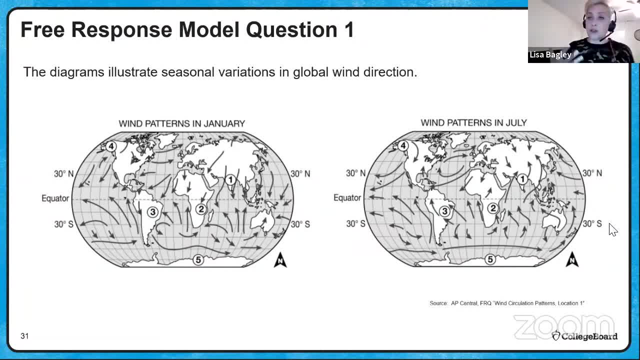 So we need to take them apart so that we can understand what is happening here and look at what the prompt is telling us and hone in on exactly what's going on. Don't get overwhelmed. Deep breath, okay. So seasonal variations in global wind direction. 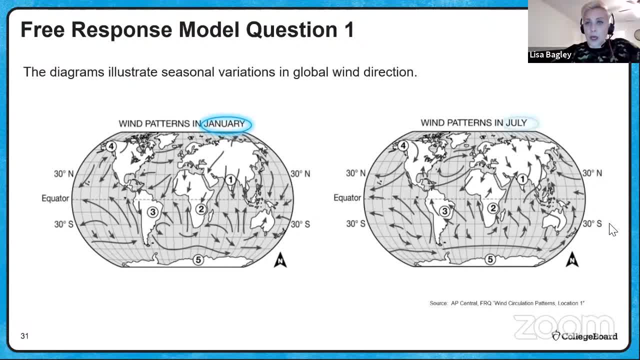 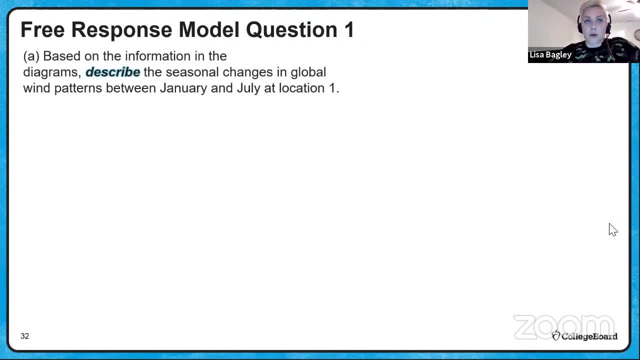 So we've got one that's for January And one that's for July. Okay, okay, We're ready to go. Question one, Based on the information in the diagrams, describe the seasonal changes in global wind patterns between January and July at location one. 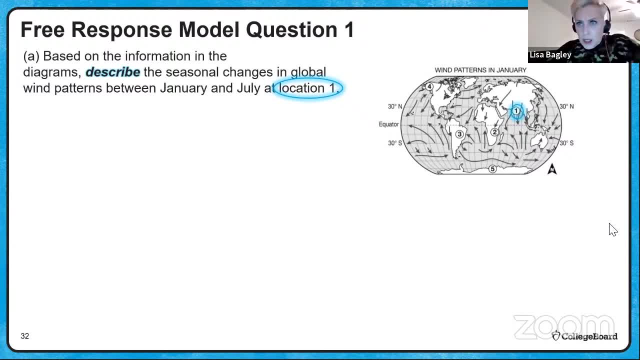 All right. so first we've got to find January, location one- All right, got it. Then we've got to find July, location one, Got it. So location one. So location one is India right, And we've got January and July. 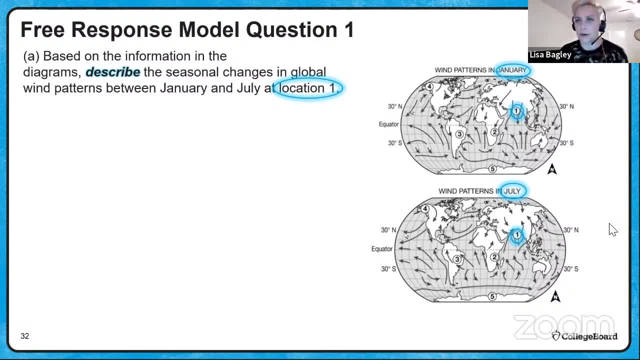 So the arrows are showing us our wind patterns. So what's going on with the winds in January? Well, they look like they're coming off the continent there, kind of out through the Deccan Plains and down into, kind of moving down from the continent down into the Indian Ocean. 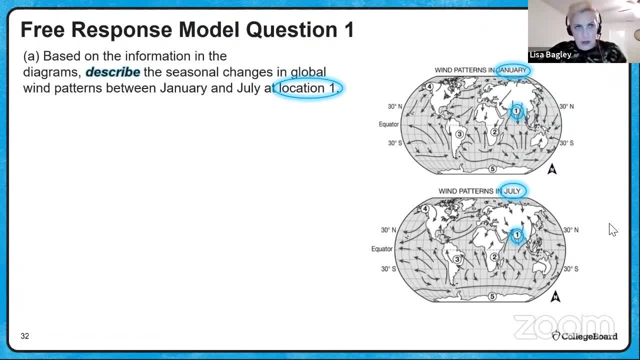 And then in July they're going the opposite way. All right, cool. So in January, the winds at location one come from the north, And in July, the winds at location one come from the southwest, And all you're doing there is describing what direction those arrows are showing. 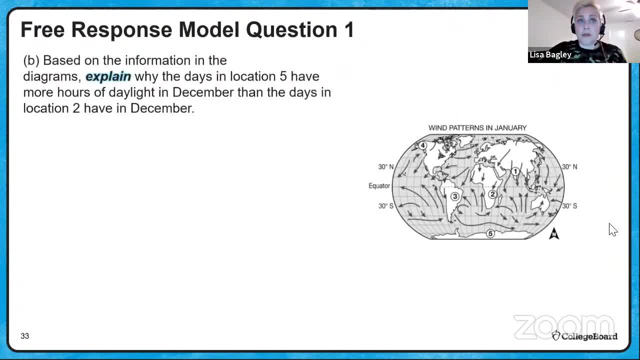 Don't get overwhelmed. All right, based on the information in the diagrams, explain why the days at location five- there it is- have more hours of daylight in December than the days in location two have in December. So we're talking December. 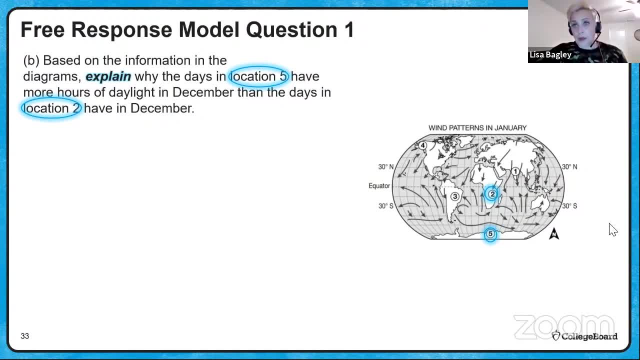 We're in the southern hemisphere. Okay, So there's our equator. December is summer in the southern hemisphere, So location five will have more hours of daylight than location two due to the tilt of the earth at that time. You could also say due to the angle of the incoming sunlight. 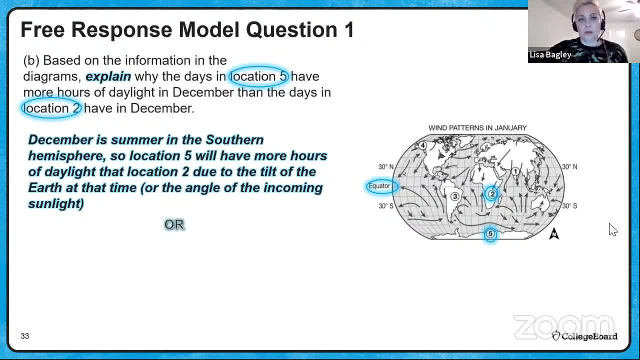 Right. So you've got to remember. in the southern hemisphere we've got our seasons reversed. Well for us in the northern hemisphere. If you're in the southern hemisphere, they're normal. Or location five is near the South Pole, where the sun never really sets during the summer, which is December for them. 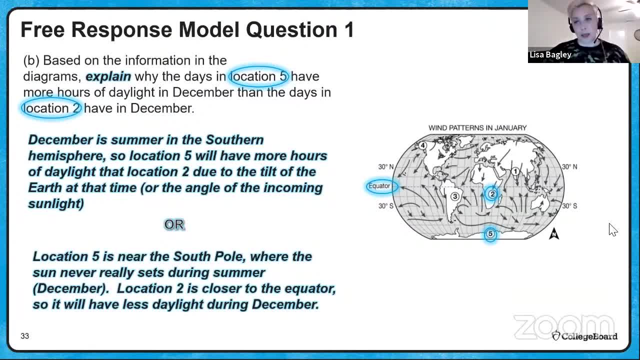 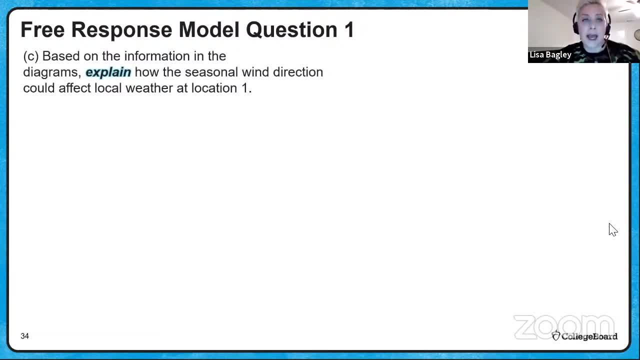 Location two is closer to the equator, so it will have less daylight during December. All right, Based on the information in the diagrams, explain how the seasonal wind direction could affect local weather at location one. So we're talking about weather, Right? 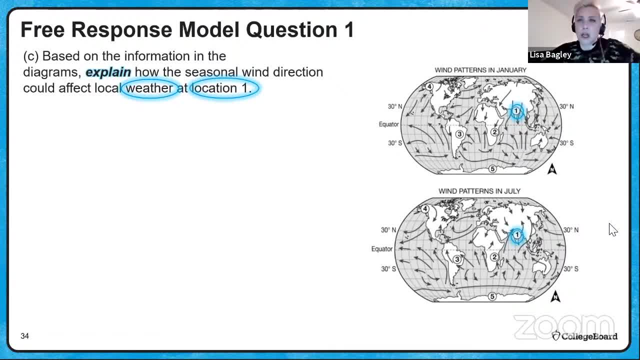 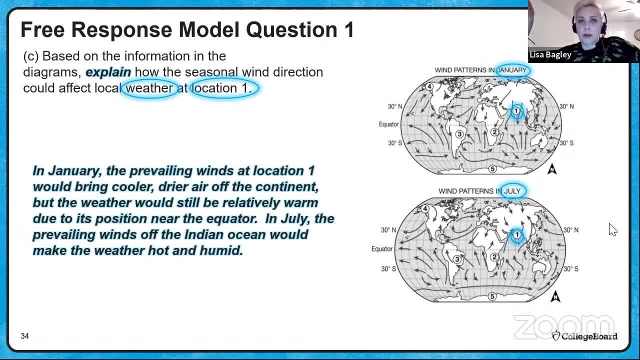 We're talking about location one, So we're back to location one, And we're talking about seasonal wind direction, So we've got to compare January and July. All right, In January the winds at location one are coming, of course, down off the continent. 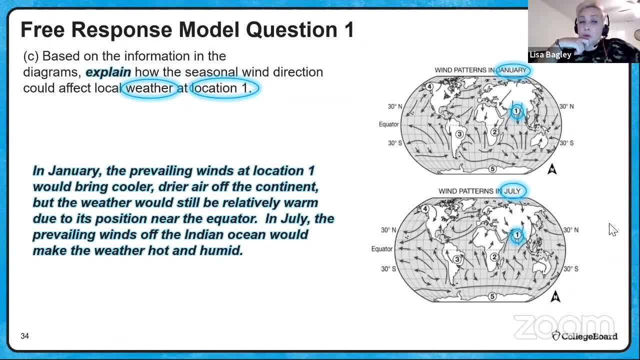 So winds coming off a continent are going to bring cooler and drier air, But this location is pretty close to the equator, So the weather will still be relatively warm because it's close to the equator. In July the prevailing winds are coming up off the Indian Ocean, which is going to make the weather hot and humid. 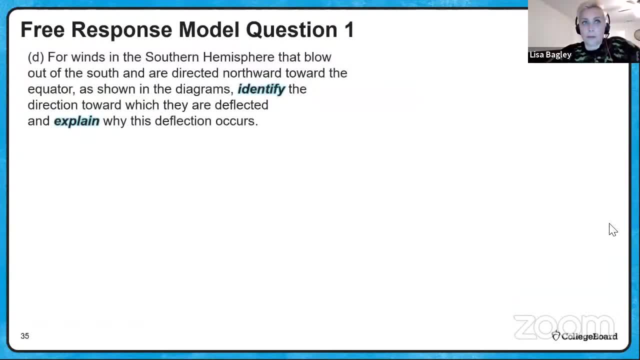 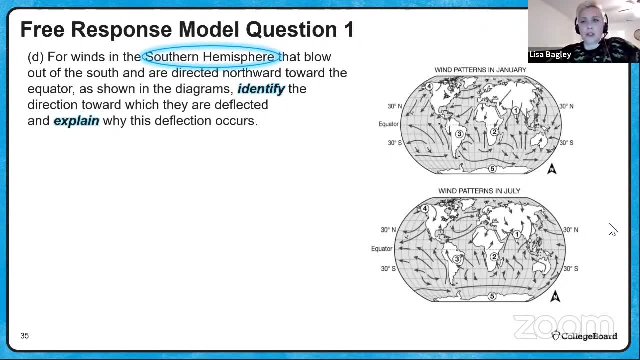 Okay For winds in the southern hemisphere that blow out of the south and are directed northward, towards the equator, as shown in the diagrams, and this is what the arrows show: Boop, Identify the direction towards which they are deflected. 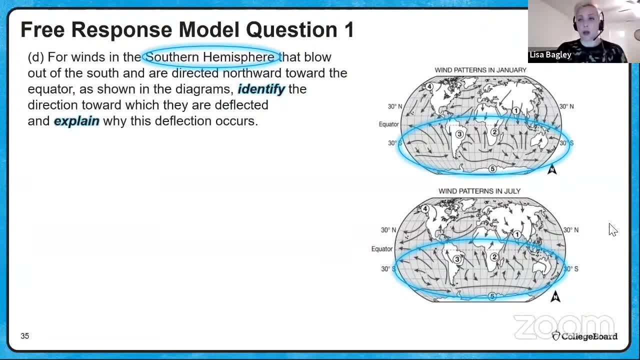 And explain the direction And explain why this deflection occurs. Okay, We're talking Coriolis effect here, So here we go. In the southern hemisphere, winds blowing northward will be deflected to the left, which is westward. 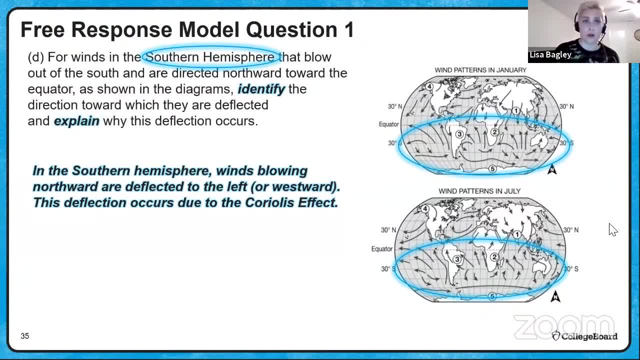 And the deflection is due to the Coriolis effect. Now do you have to describe the Coriolis effect? Nope, You have to explain why the deflection occurs. And it is the result of the Coriolis effect, which is that deflection is due to the earth spinning on its axis. Every few years in the southern hemisphere, the winds over the Pacific Ocean, as shown in the diagrams, weaken or reverse direction, Describe the typical change to the weather pattern that happens along the northwestern coast of South America during those years. So if you've been following along, this is going to be an El Nino question. 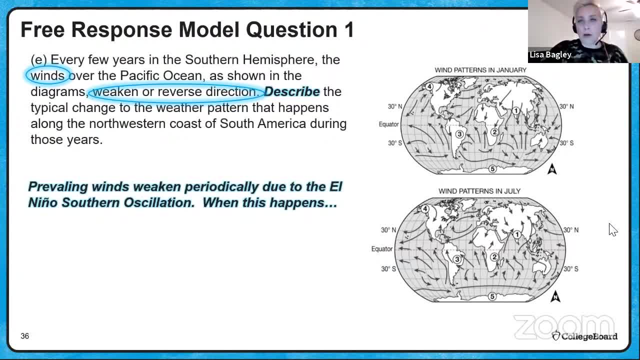 So first orient yourself on the map Right. So we're talking about the coast, The northwestern coast of South America, And I had mentioned that those prevailing winds weakened or reversed direction. So prevailing winds weaken periodically due to the ENSO, the El Nino Southern Oscillation. 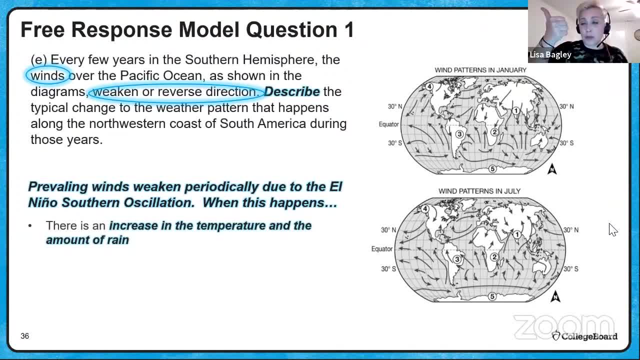 When this happens, there's an increase in the temperature and the amount of rain, because the surface temperature of the water stagnates and increases. The weather is warmer and there are more storms. There can be major flooding in parts of South America, which sometimes leads to pretty severe weather. 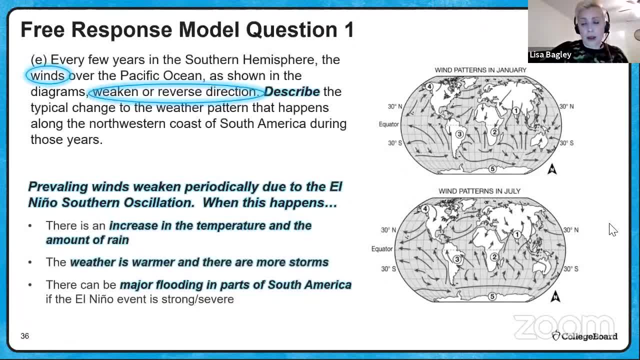 All right. So any of those right, you're going to kind of describe what happens during an El Nino Southern Oscillation event. So again, you might want to go back and take a look at that in your content. All right. 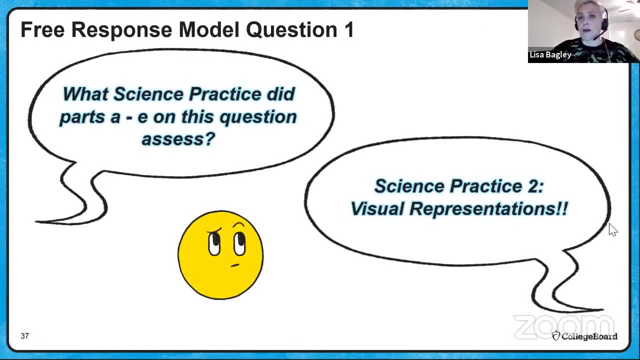 All of these parts that we just went through A through E, are visual representations. They are based on analysis of a map that you are taking a look at And again, this is unit four is visual representations. Unit four is visual representation: heavy. 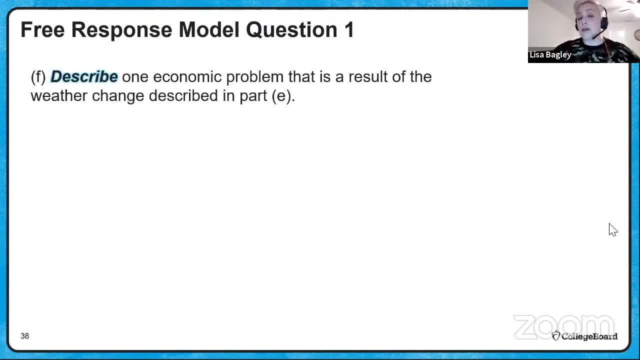 All right, So describe an economic problem that's the result of the weather change that you described in part E. So what's an economic problem that happens due to El Nino? This is concept explanation. Since El Nino events cause warmer weather and heavy rains in coastal South America and they reduce cold water upwelling along the coast, any of the following economic issues could occur. 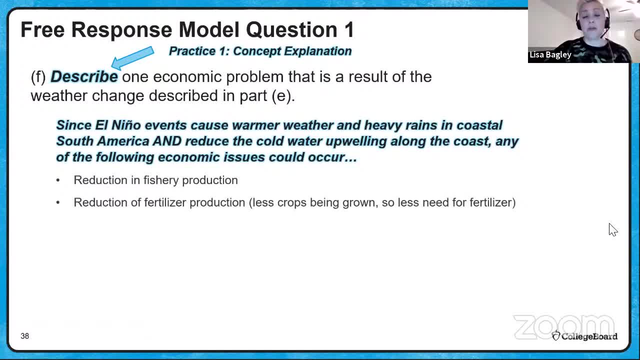 We could have a reduction in fishery production. We could have a reduction in fertilizer production, Like what? Well, less crops are being grown, so less need for fertilizer. We could have property damage from flooding or property damage from landslides. 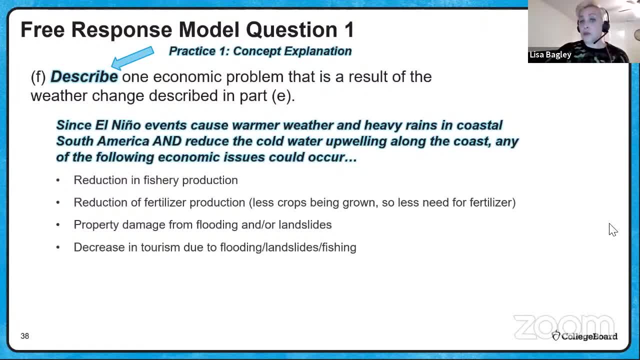 There will be a decrease in tourism because of flooding, landslides or maybe just a lack of the fishing We might have damage to crops from extreme weather. Any of those could be economic issues. Finally, Increased healthcare costs or loss of productivity, meaning that people aren't working, from the spread of vector-borne or water-borne infectious diseases. 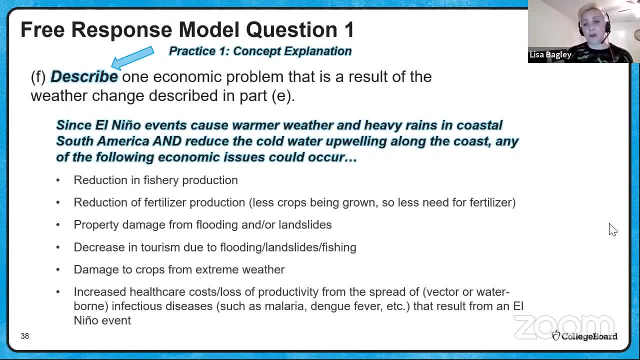 If the water is stagnant, you're going to have more malaria, dengue fever or any warmer water-borne diseases. They would increase in this area. All right, Identify a characteristic of the expected climate On the slope of a mountain. 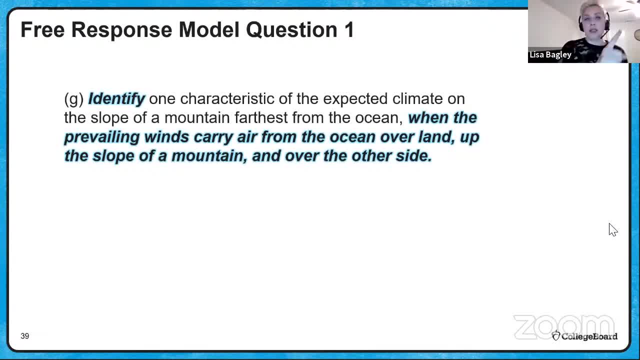 Farthest from the ocean, When the prevailing winds carry air from the ocean over land, up the slope of a mountain and down over the other side, Rain shadow. They literally described it for you. Okay, So the expected climate on the slope of a mountain furthest from the ocean will be cooler and drier. 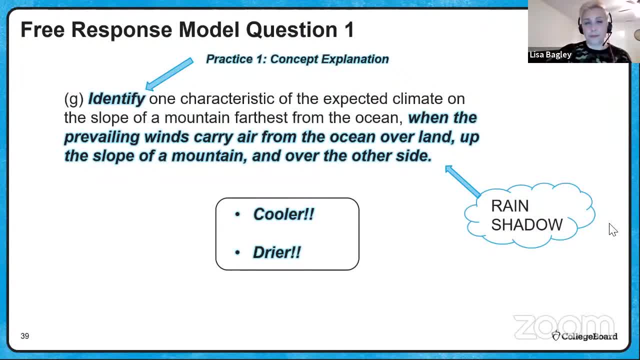 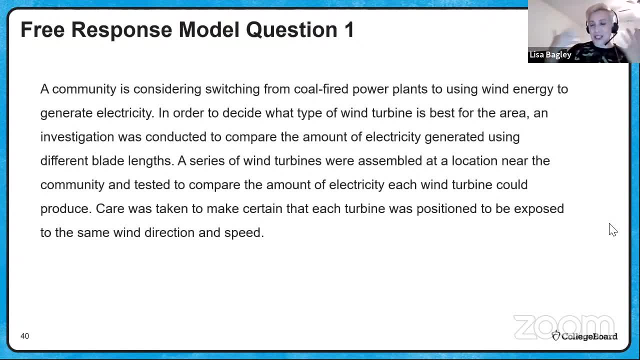 That's the definition of the rain shadow. Okay, Finally, A community is we're heading over here to experimental design. A community is considering switching from coal-fired plants using wind energy to generate electricity. In order to decide what type of wind turbine is best for the area, an investigation was concluded or conducted to compare the amount of electricity generated using different blade lengths. 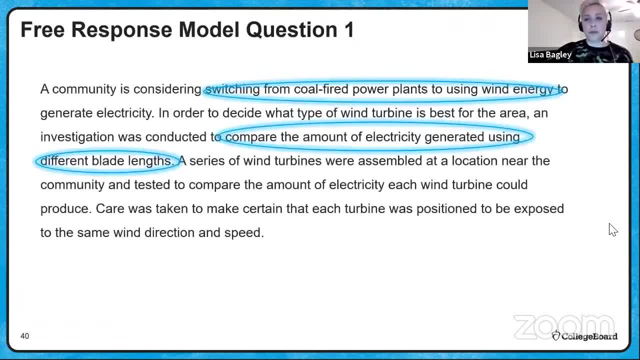 A series of wind turbines were assembled at a location near the community and tested to compare the amount of electricity each wind turbine could produce. Care was taken to make sure that each turbine was positioned to be exposed to the same wind direction and speed. So those are our constants. 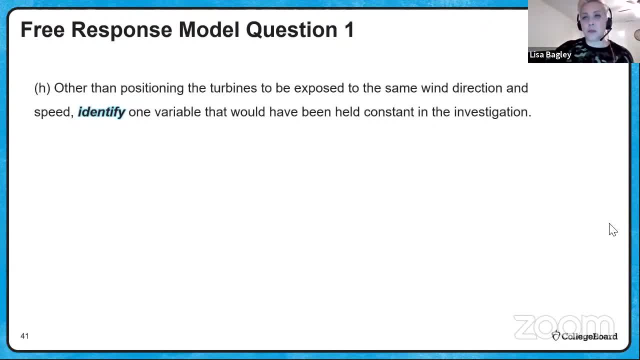 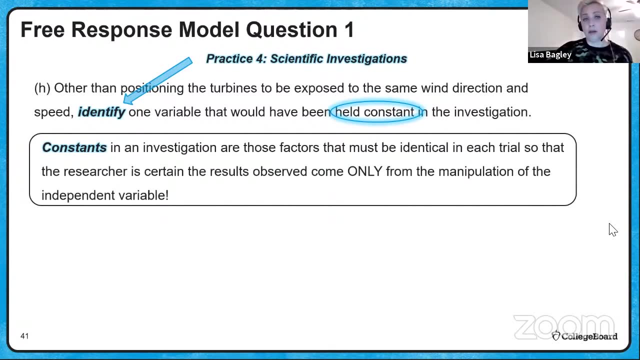 All right, Other than positioning the turbines to be exposed to the same wind direction and speed, identify a variable that would have been held constant in this investigation. All right, Again, here we are, in practice four. Remember that constants in an investigation are the factors that must be identical in each trial, so that the researcher is certain that the results observed come only from the same wind direction and speed. 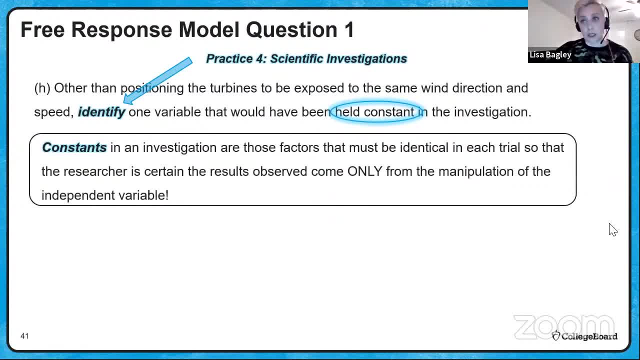 Okay, All right. Another variable is the height of the turbine, The material of the turbine, the number of the turbine blades, the width of the blades, the angle or the pitch of the blades and the duration of the test. All of these must be held constant, or you can't be sure that you're getting results from what you think you are. 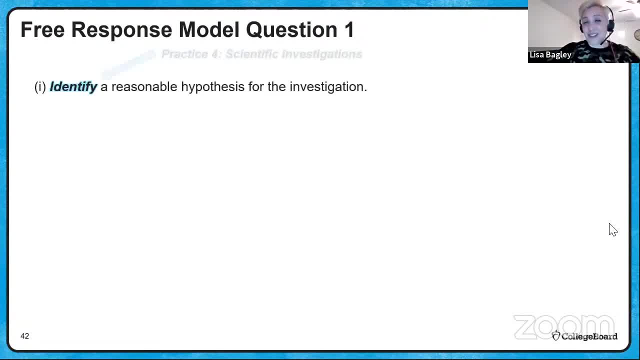 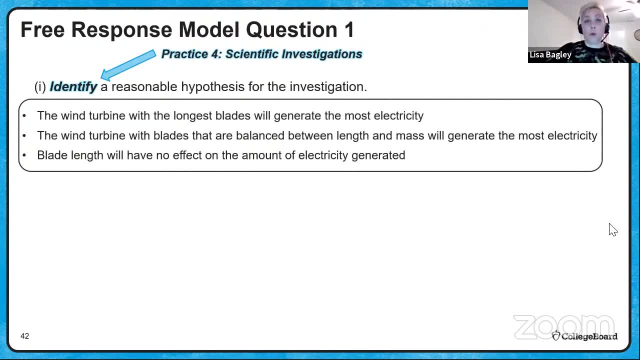 Okay, Identify a hypothesis for the investigation. Okay, The wind turbine with the longest blades will generate the most electricity, Or the wind turbine with blades that are balanced between length and mass will generate the most electricity, Or blade length will have no effect on the amount of electricity generated. 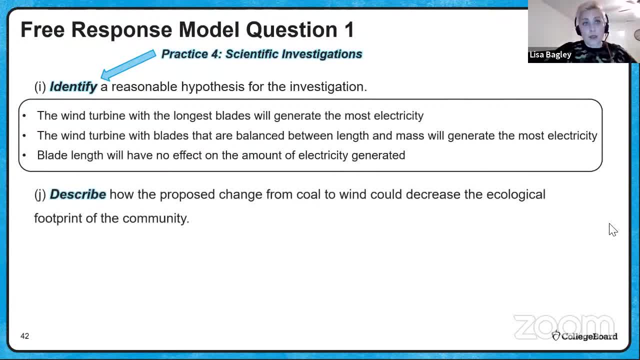 Null hypothesis is always fine. Describe how a proposed change from coal to wind could decrease the ecological impact. Okay, The wind turbine would reduce the ecological footprint of the community. All right, So ecological footprints are topic 5.11.. We've asked about these several times in the past. 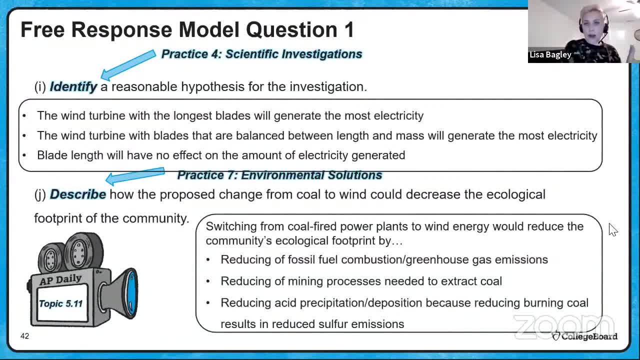 So good to review it. So switching from coal-fired power plants to wind energy would reduce an ecological footprint by reducing the fossil fuel combustion or greenhouse gas emissions. Reducing the mining processes needed to extract coal, Reducing acidic precipitation or deposition Reduction of burning coal results in reduced sulfur emissions. 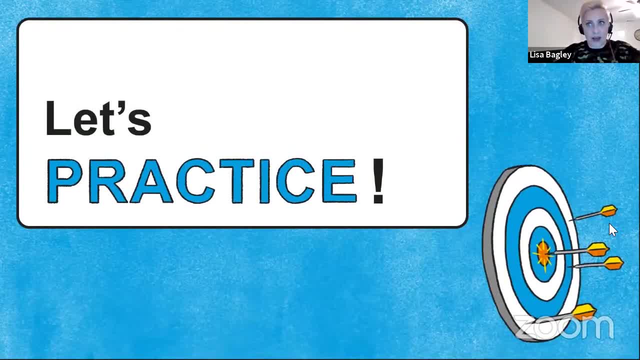 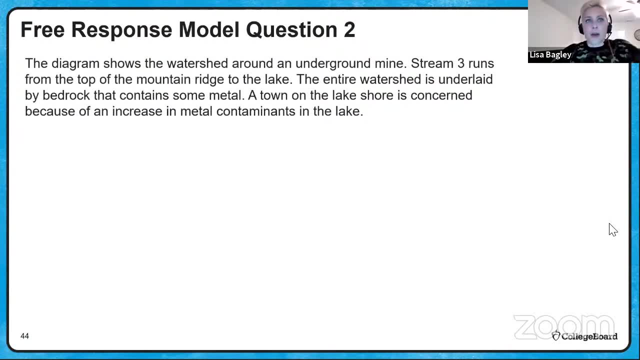 All right, So we're going to go a little faster through the second one. You kind of got the idea, And this one is fairly similar in the terms of how it's structured. Here we go. It's a diagram. It shows a watershed around an underground mine. 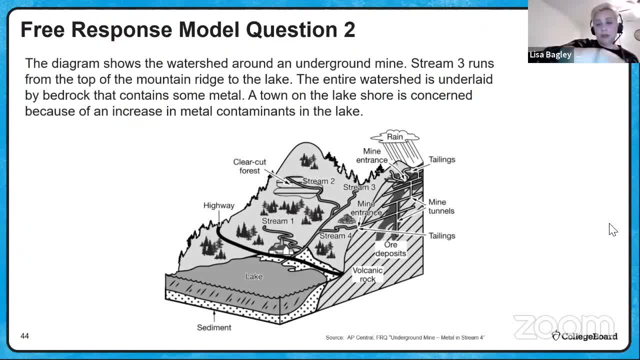 Stream 3 runs from the top of the mountain down to the lake. The entire watershed is underlaid by bedrock that contains some metal. There's a town on the lake shore That's concerned because there's an increasing amount of metal contaminants in the lake. 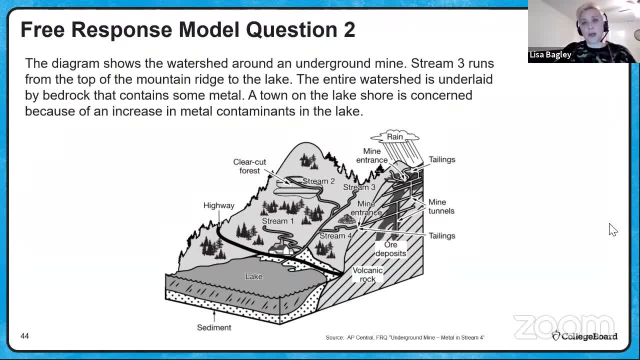 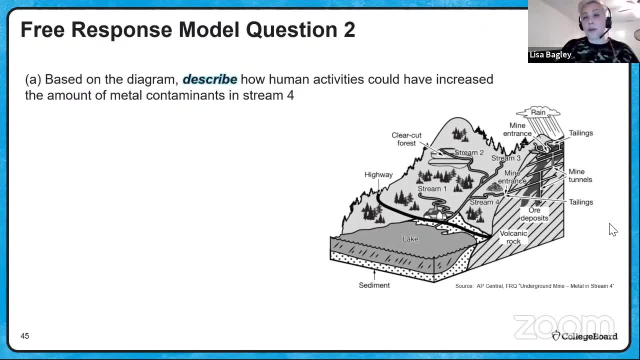 Again, this is a very detailed visual model and we're going to take it apart. All right, Here we go. Based on the diagram, describe how human activities could have increased the amount of metal contaminants in stream 4.. So, first off, let's find stream 4.. 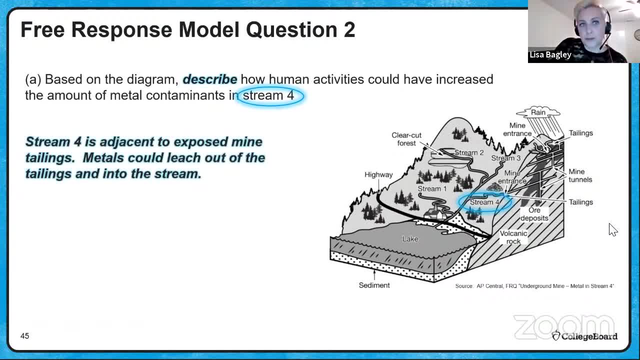 There it is Okay. Notice that it's close to the mine. Stream 4 is adjacent to the mine And exposed mine tailings, which you see there in the picture. The metals could leach out of the tailings and into the stream. 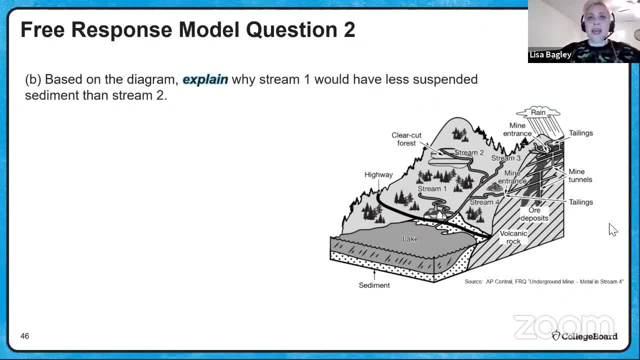 Okay, Same diagram that we're working on Explain why stream 1 would have less suspended sediment than stream 2.. First off, let's orient ourselves. There's stream 1. And there's stream 2.. All right, So stream 1 has an intact forest next to it. 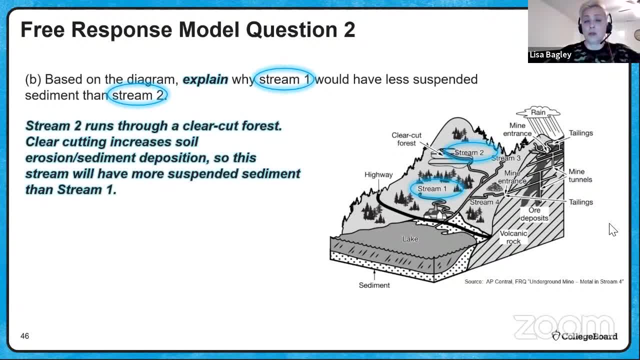 And stream 2 has a clear-cut forest. Stream 2 runs through a clear-cut forest. Clear-cutting increases soil erosion and sediment deposition, So the stream is going to have more suspended sediment than stream 1.. But stream 1 also meanders more. 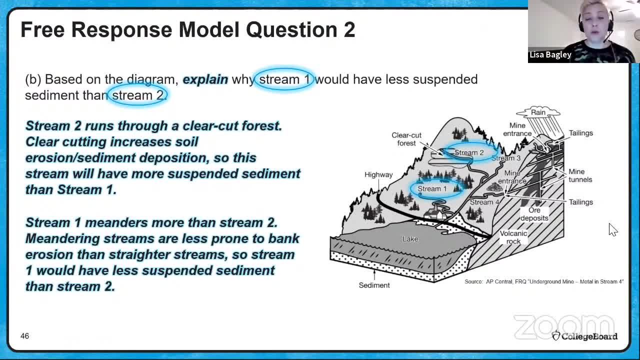 The word meander means to weave back and forth. Stream 1 meanders more than stream 2.. And meandering streams are less prone to bank erosion than straighter streams. So stream 1 might have less suspended sediment than stream 2 due to that. 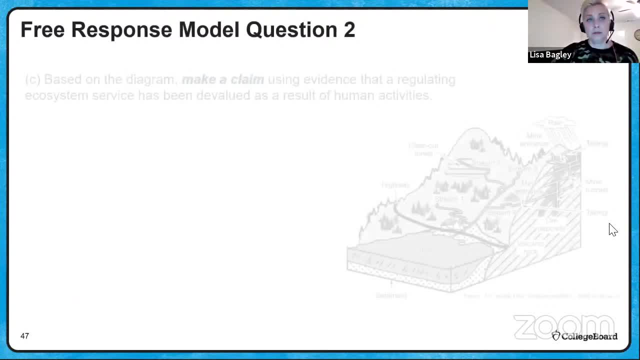 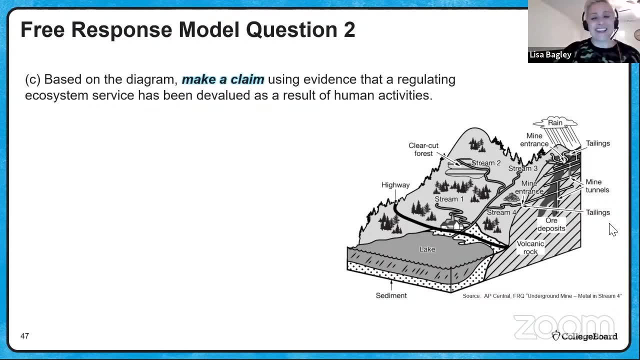 Either one of those are acceptable. Same diagram: Different prompt: Based on the diagram, make a claim Using evidence that a regulating ecosystem service has been devalued as the result of human activities. Now, we modeled this in the beginning, So here we go with the actual model that you can see. 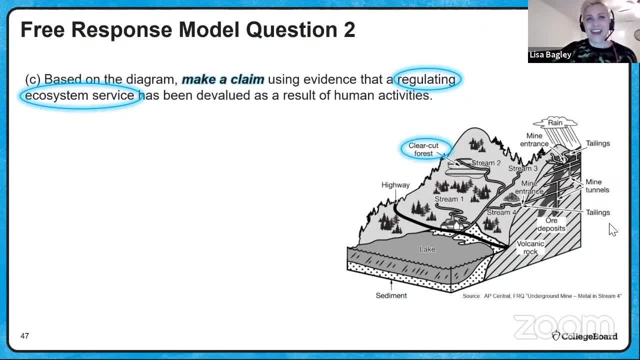 So we need a regulating ecosystem service, Right, And we need to talk about the devaluation of that. So, when we look at this diagram, the best choice for this answer right is our clear-cut forest. This is topic 2.2, which is regulating ecosystem services. 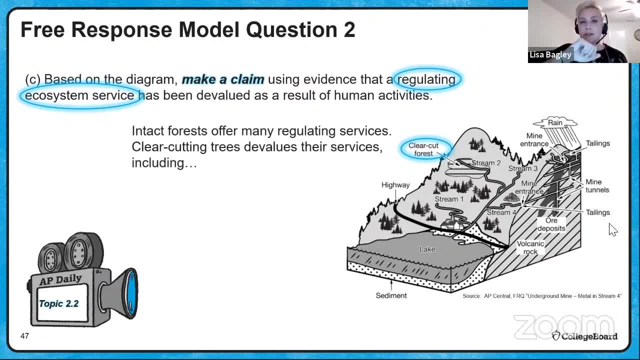 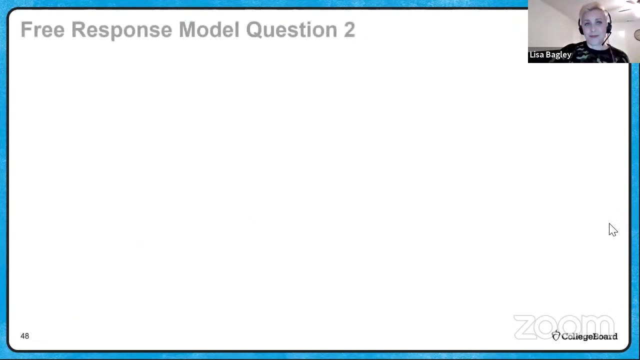 So intact forests offer many regulating services. Clear-cutting trees devalues those services, And these include erosion control, filtration of air and water, flood control, carbon sequestration or pest mitigation. So when you clear-cut a forest, you devalue its regulating service. 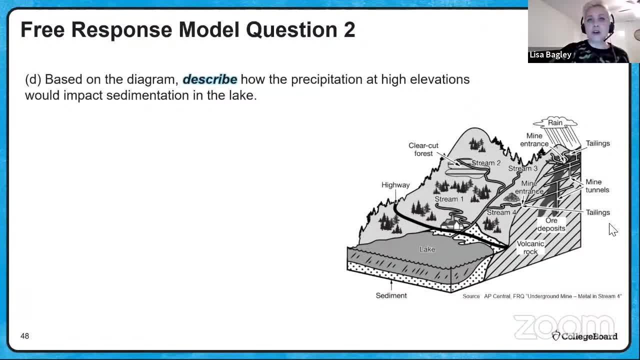 Same diagram, Different prompt Describe how the precipitation at high elevations would impact sedimentation in the lake. So here's our rain up at high elevations Lake is down below. What's going to happen when it rains up top down in the lake. 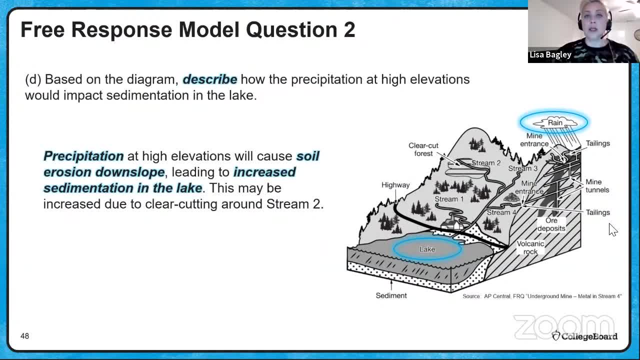 Well, precipitation at high elevations will cause increased soil erosion downslope Right, Which is going to lead to increased sedimentation down in the lake, And this actually may be. this process may be increased due to the clear-cutting that you see around stream 2.. 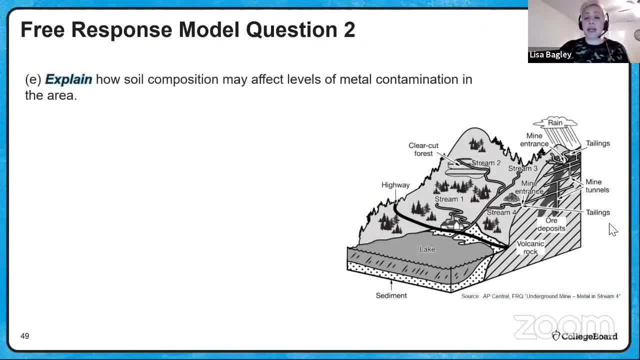 Explain how soil composition may affect levels of metal contamination in the area. Now caveat: when you look at this diagram here, they don't tell you anything really about the soil composition in the area, So you have to kind of go with what you know about soil composition. 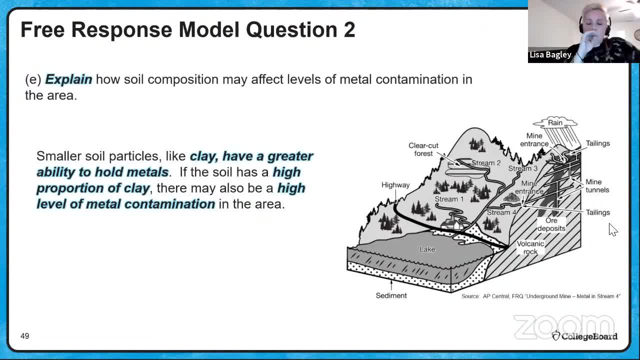 Here. So smaller soil particles like clay have a greater ability to hold onto metals. So if the soil has a high proportion of clay, which you don't know, based on this diagram there may also be a higher level of metal contamination in the area. 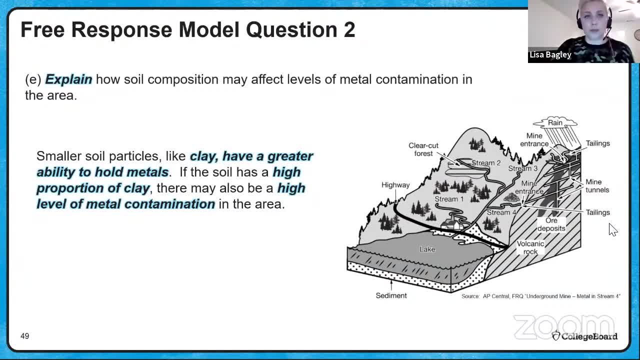 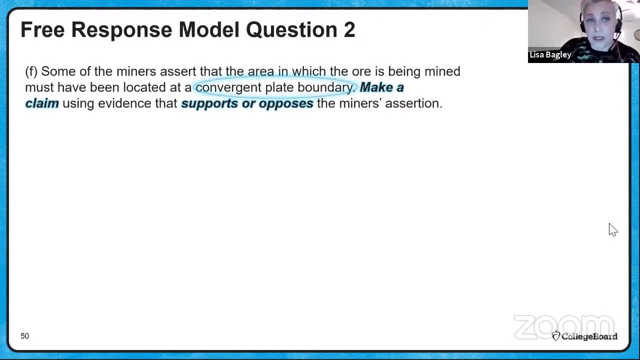 So this is based on what you already know about soils. Some of the miners assess assert that the area in which the ore is being mined must have been located at a convergence point. So if the soil is located at a convergent plate boundary, make a claim using evidence from the diagram that supports or opposes the miner's assertion. 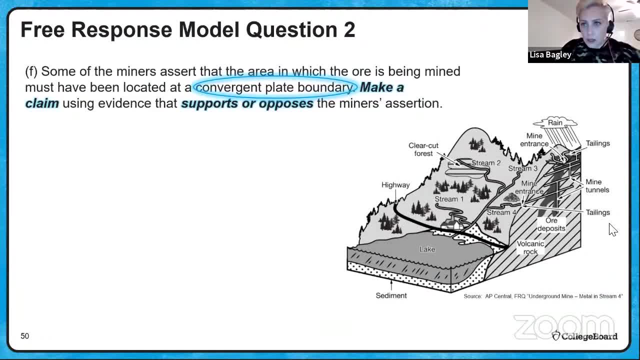 Okay, There's our same visual prompt. Okay, Let's take a look. Well, if you're going to support the miner's claim, you can see that there's volcanic rock right there in the visual. Volcanic rock can form at a convergent plate boundary. 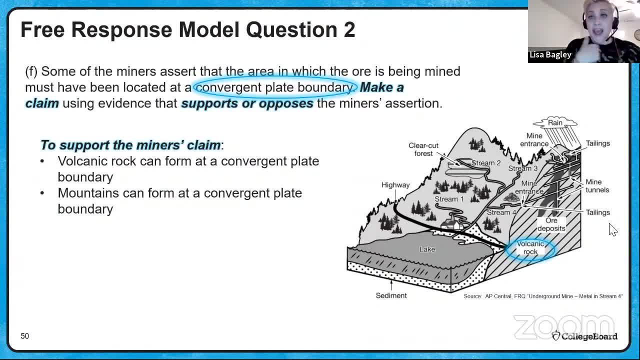 Because we said, volcanoes of course are a feature Convergent plate boundaries And notice that there's an elevation change there, So mountains can also form a convergent plate boundary. So you do have evidence of that in the graph. 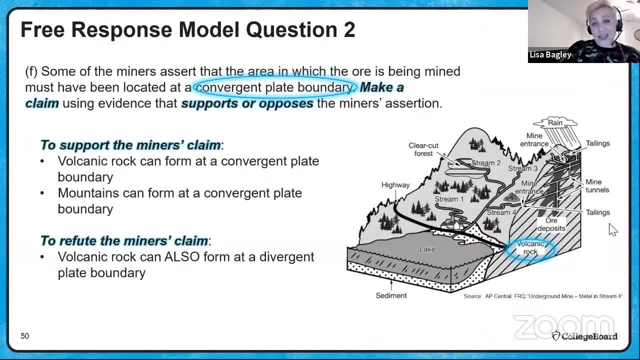 But you could also refute the miner's claim Because you know what Volcanic rock can also form at a divergent plate boundary. So you can give evidence from the graph for either supporting or refuting the miner's claim. All right, 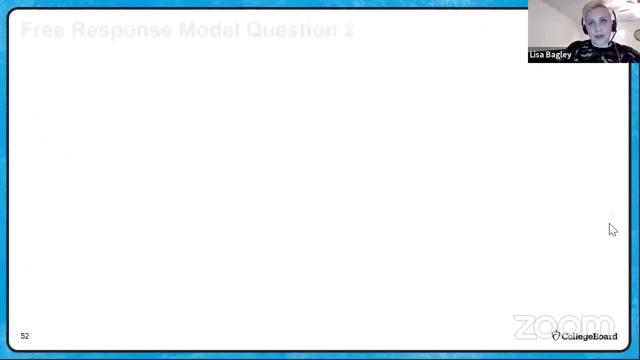 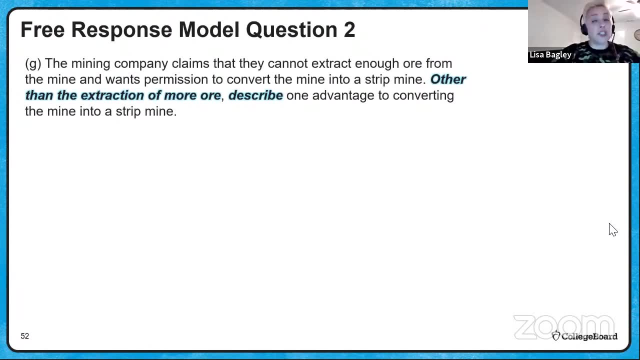 A through F. here Again visual representations, And that's pretty heavy in this unit. All right, The mining company claims that they cannot extract enough ore from the mine and wants permission to convert the mine into a strip mine. Other than the extraction of ore, describe an advantage to converting the mine into a strip mine. 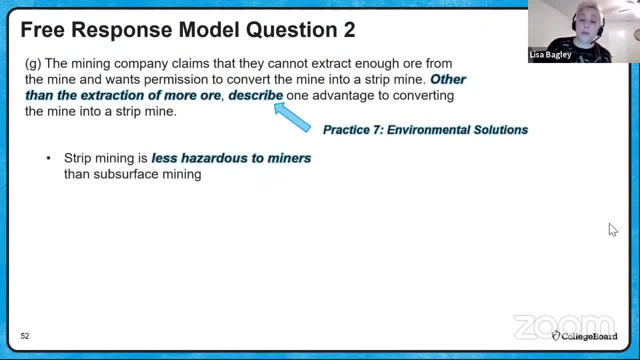 Hmm, Okay. Well, strip mining is less hazardous to miners than subsurface mining. People don't have to go underground, They don't have to breathe coal dust- Less hazardous. Strip mining is less expensive than subsurface mining due to labor costs, healthcare costs for miners and increased efficiency. 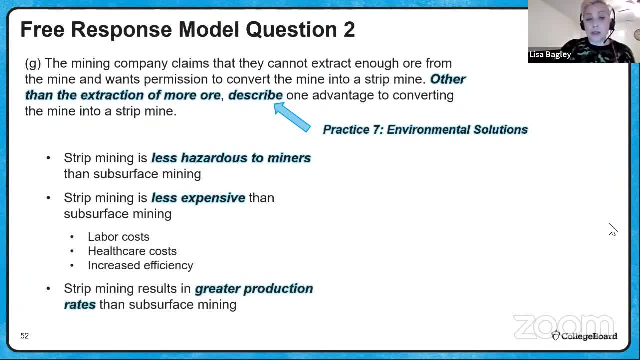 Strip mining results in greater production rates than subsurface mining, And any of those would be evidence right for describing an advantage to converting your mine- the subsurface mine that you see in the diagram- into a strip mine. All right, Last little bit here. 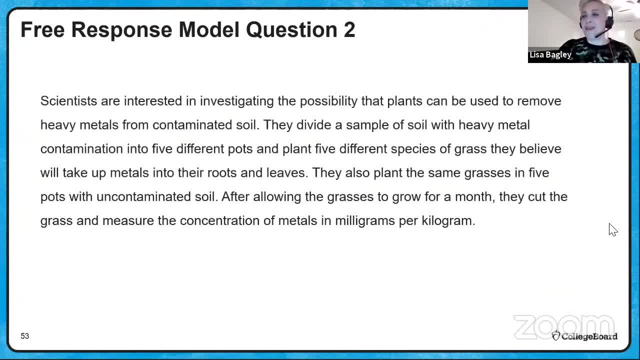 And that, of course, is our experimental design. Scientists are interested in investigating the possibility that plants can be used to remove heavy metals from contaminated soil: Phytoremediation: They divide a sample of soil with heavy metal contamination into five different pots and plant five different species of grass they believe will take metal up into their roots and leaves. 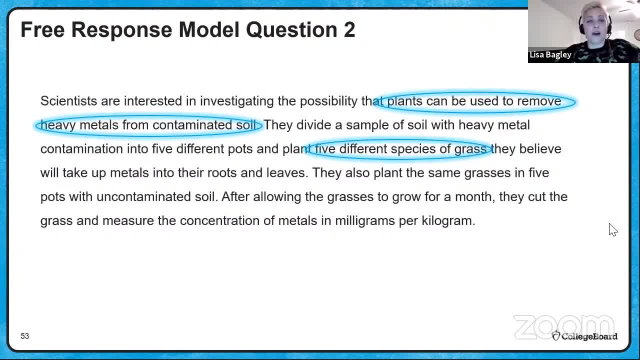 They also plant the same grasses in five pots with uncontaminated soil, So that's a good example. After allowing the grasses to grow for a month, they cut the grass and then measure the concentration of metals in milligrams per kilogram. 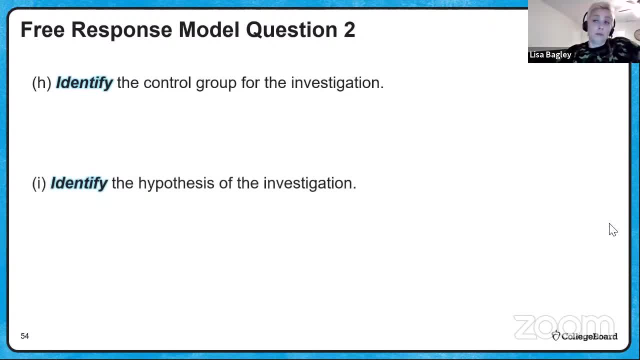 What's the control And what's a valid hypothesis? Those are both scientific investigation questions. So remember that the control group is going to be the group that's closest to the normal conditions or receives no treatment, And that, of course, would be the group of plants growing in the uncontaminated soil. 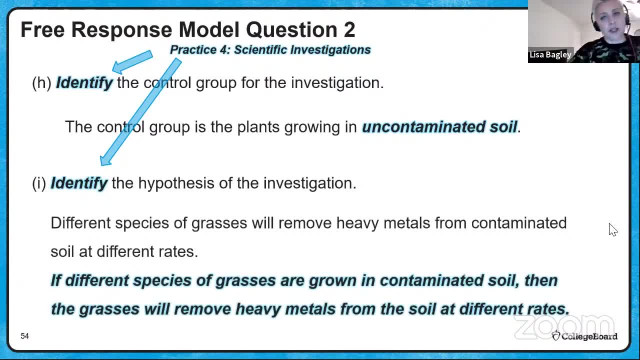 A good hypothesis for the investigation. I want to model this really quickly. You could say different species of grasses will remove heavy metals from contaminated soil at different rates. But if you want to put it in an if-then I gave this to you too. 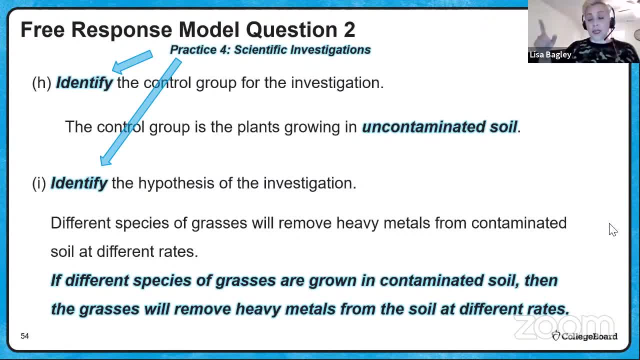 If different species of grasses are grown in contaminated soil, then the grasses will remove heavy metals from the soil at different rates. Do you have to do if-then? No, But if you're used to doing that in your science classes, that's a way to take that answer and model it in if-then. 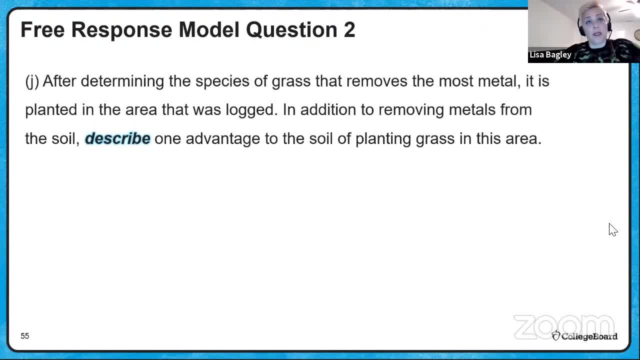 Finally, after determining the species of grass that removes the most metal, it is planted in the area that was logged, In addition to removing metals from the soil. describe an advantage to the soil of planting grass in the area. Well, when you plant grass, you decrease soil erosion. 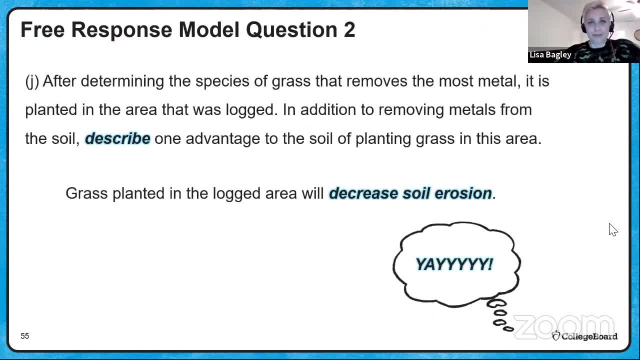 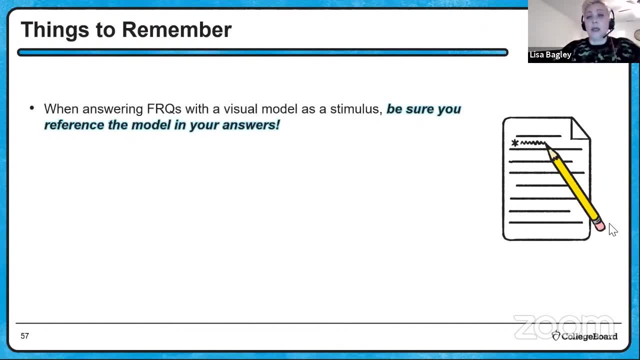 Easy peasy, Yay, All right. So what should we take away? Things to remember: When answering free response questions with a visual model as a stimulus, you must be sure to reference the model in your answers. As you read a prompt with an experimental setup, determine the independent and the dependent variables, even if the question doesn't ask you to identify these. 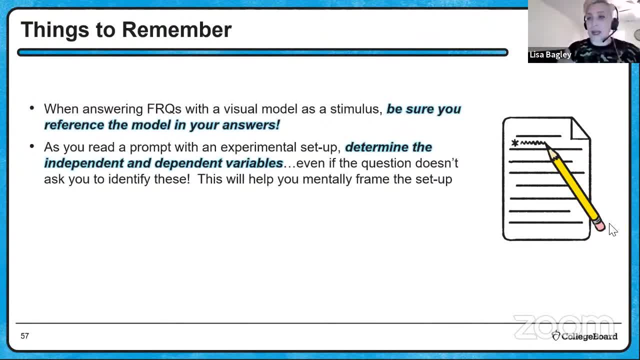 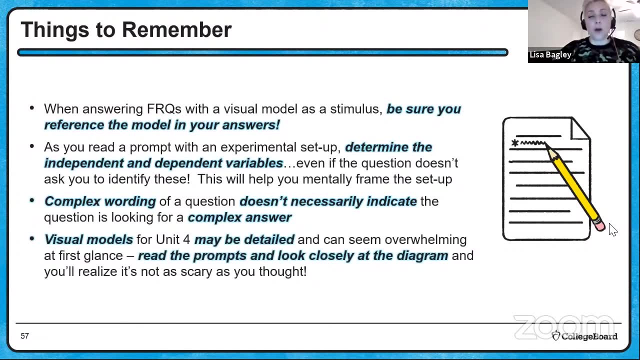 Because this is going to help you mentally frame the setup of the experiment. Complex wording of a question doesn't necessarily indicate that the question is looking for a complex answer. So take it apart. Visual models for Unit 4 may be detailed and they can seem overwhelming at first glance. 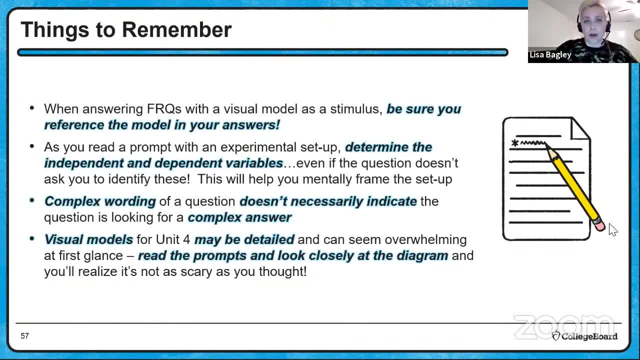 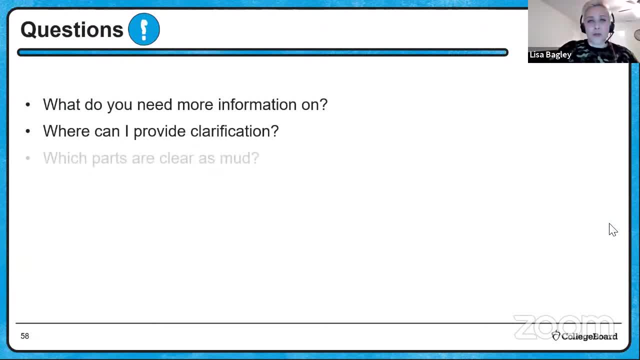 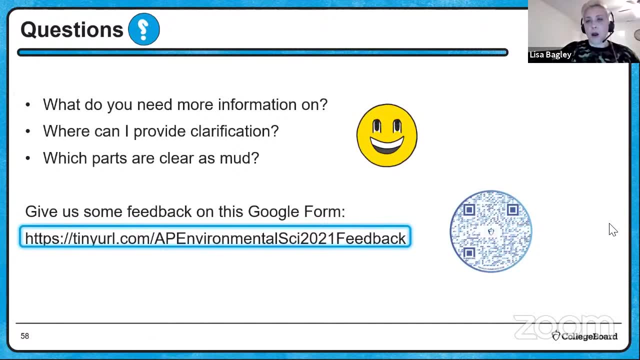 Take a breath, read the prompts and look closely at the diagram and you'll realize they're not as scary as you think. All right Questions. Where can I provide more information, clarification and all that good stuff? Here's our wonderful Google feedback form and your QR code for that. 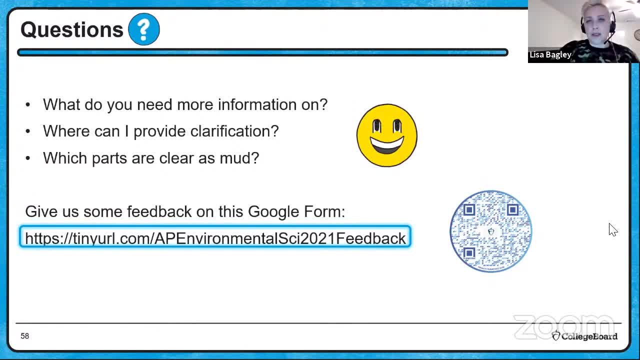 I'm always, always interested in your feedback. It makes things better and I love to answer your questions. And again, of course, you might get a shout out at the beginning of next video, So be sure to tune in Daily video 4 preview. 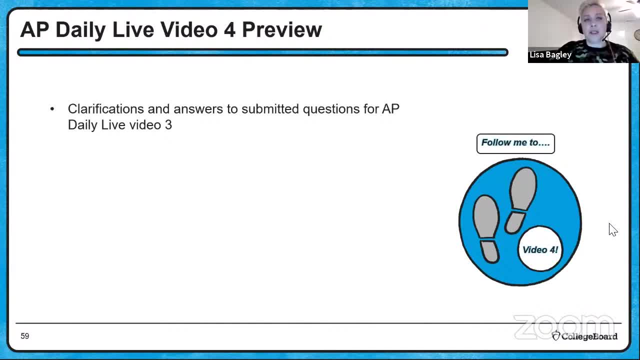 We're going to have clarifications and answers to submitted questions for AP Daily Live video 3,, which was today. Content review for land and water use, Which is Unit 5.. Free response modeling focused on connecting content knowledge with our science practices, which we've been doing all week. 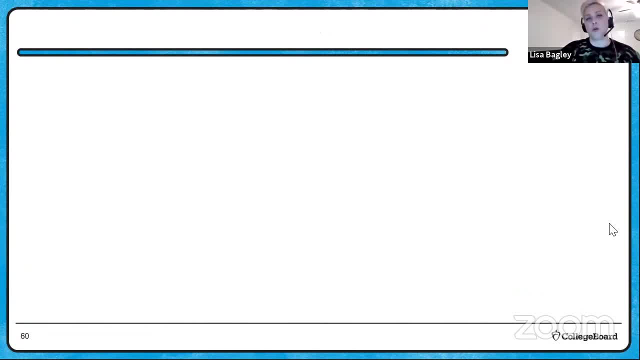 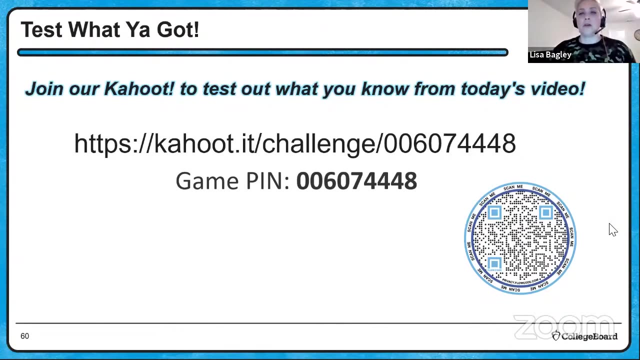 And interactive practice on concepts in video 4.. So join our Kahoot to test out what you know from today's video. Test what you got folks, There's your Kahoot link and your QR code. Today's game pin is 006074448.. 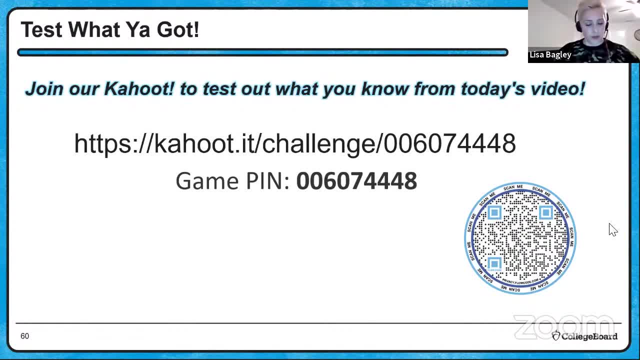 Let's see how you do. Let me give that to you for a sec. Let you grab it, All right. Thanks for watching everybody, And I'll see you tomorrow. Bye-bye.